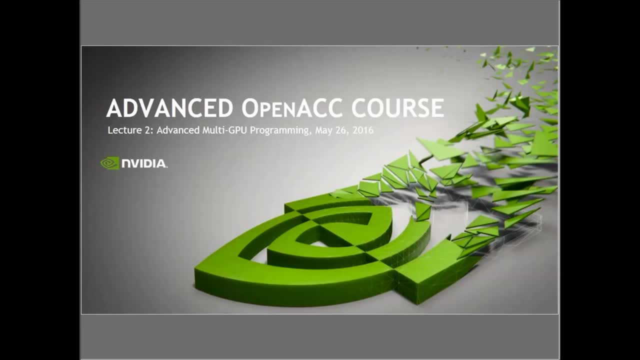 Thanks for joining the lecture today. Today is going to be our last lecture of the course And my name is Julia Levitas. I'm a product manager at our Tesla Group and will help with the class today, So we have changed the structure of the course a little bit since the last time. We decided to make the session today a little bit longer than usual, So it's going to be an hour and a half long and we will be able to answer more questions today. 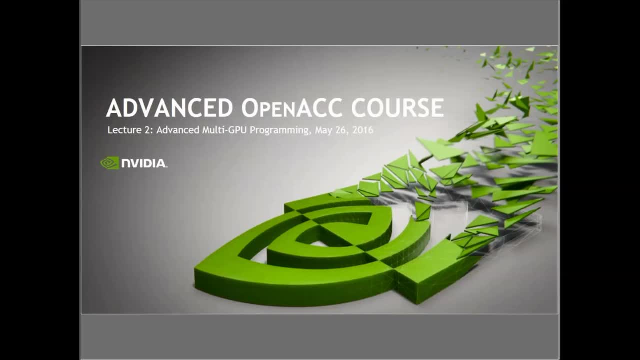 So the long lecture today was 30 minutes. For our Q&A we'll replace the office hour next week. So today is the last session of the course And we will definitely do more courses and we'll keep you posted on their new announcements. 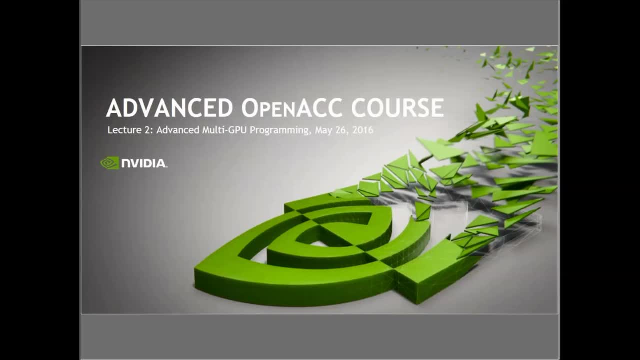 So let's start with some logistics. So every session of the course will be recorded and available for you to review on our OpenACC course page. So again to find it, you can just Google Advanced OpenACC course and the first page in the search that will show up will be the page for the course. 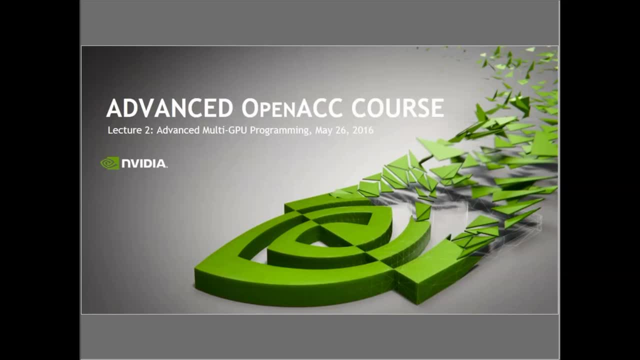 We'll be posting there all the recordings All again. you can find the Q&A and the slides, So probably tomorrow you will be able to find those on the page. So all the lines are muted right now. So please submit your questions through the Q&A pod on the right hand side or the bottom of the screen. We'll do our best to answer as many questions as we can. today especially, we have this long session. But also keep in mind we do have an email address that you can send your questions to is openaccnvidiacom, So that's a source that you can use for your help. 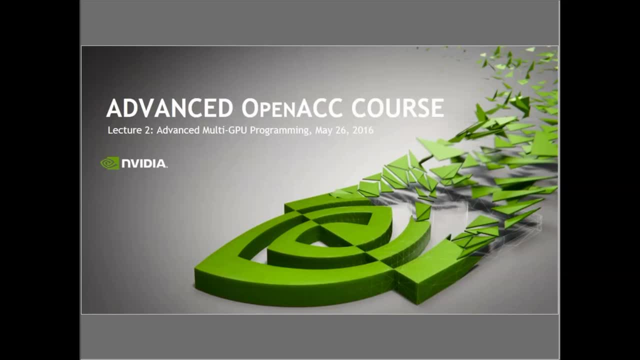 We also monitor the Stack Overflow, so you can use this form as well. And with that I believe we're done with the announcements, And I would like to introduce you to our instructor today. Jerry Krause is a Dev Tech at NVIDIA who is a goer in OpenACC and Multi-GPU topics, among a lot of others, And he's working with GULIC Supercomputer Center helping them accelerate HPC applications. 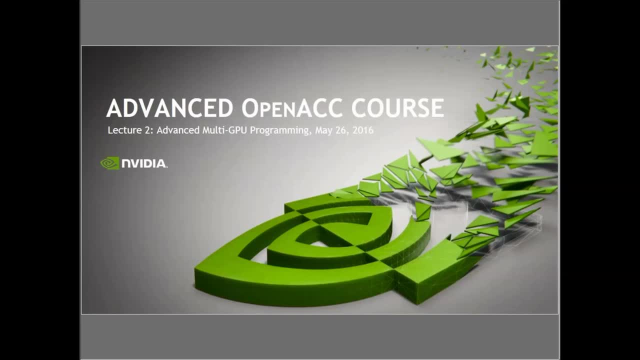 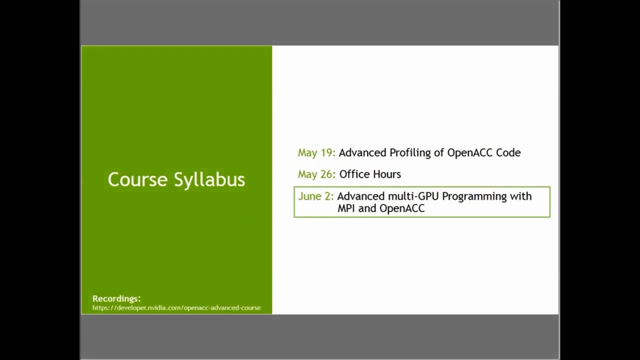 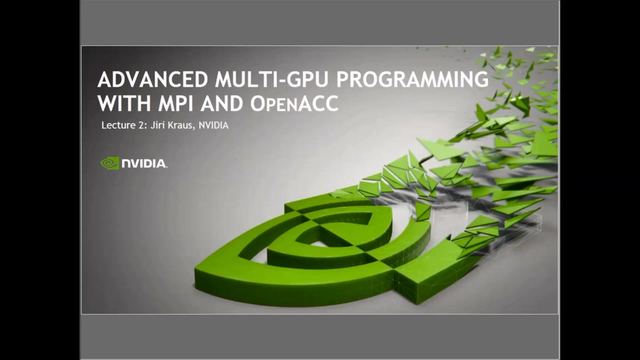 Jerry, are you ready? Yes, thanks for the introduction And also welcome from me to everybody on the course. Thanks for joining. Yeah, I will talk about Advanced Multi-GPU Programming with MPI and OpenACC. For those of you who have been joined the last online course, there's a little bit of overlap because I reintroduced some aspects. 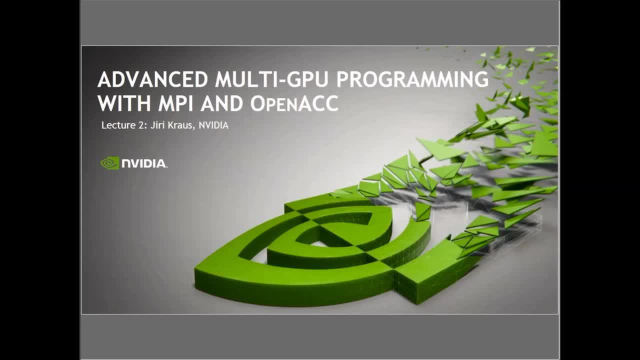 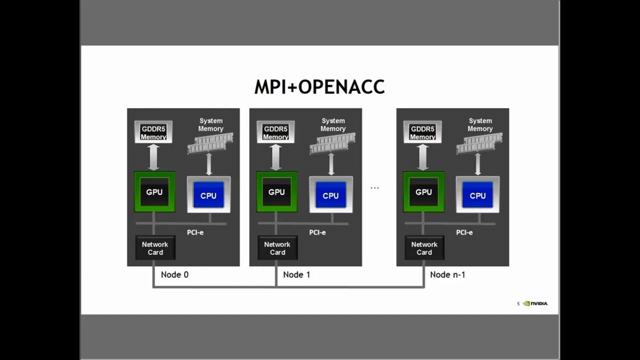 Okay, So I'd like to give a very quick introduction to what MPI and what Multi-GPU Programming with MPI means in general, so that everybody can catch up. So let's get started. So MPI plus OpenACC Programming is interesting for you because you probably want to program multiple GPUs in a cluster distributed, in this case, of N nodes. 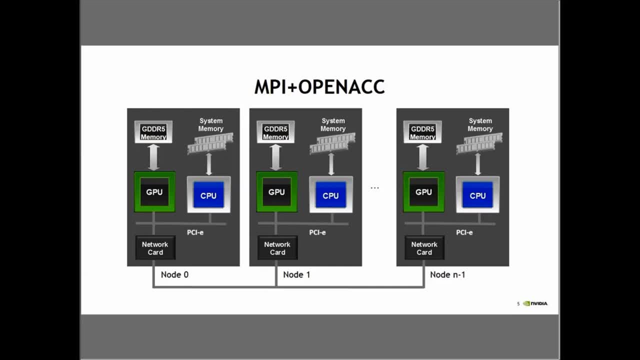 Each node has one GPU And if you want to use that cluster to solve a program coordinatively so that you'll reach the solution faster, you'll probably need to exchange messages at some point, So sending data from the GPU memory, for example from node 0, to the memory of the GPU in node N-1.. 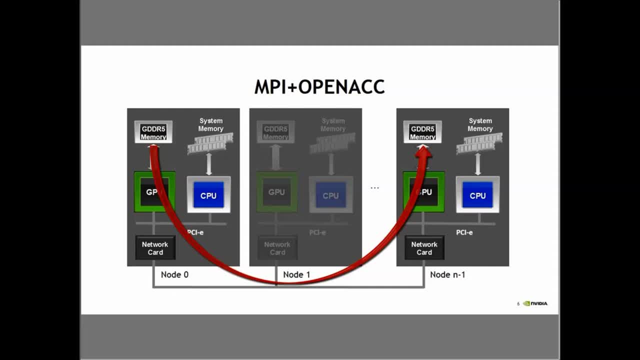 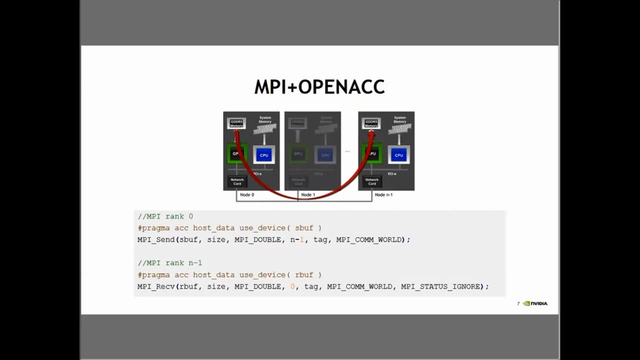 And if you know MPI and OpenACC already, that is fine. It essentially really works as expected. You just call MPI- send on the device on the buffer in the GPU of node 0, and MPI- receive on the buffer in node N-1.. 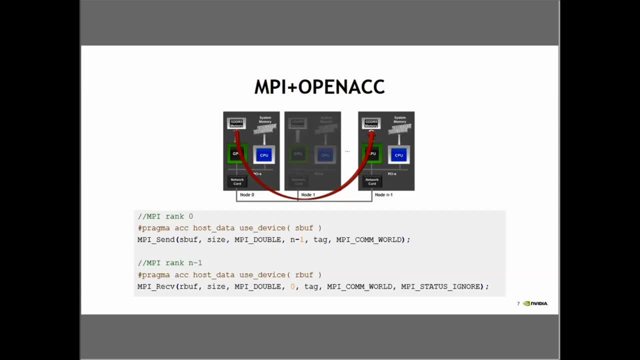 For that it's important that you use ACC host data use device because per default the OpenACC compiler would pass in the host representation the host reference of a buffer and not the device, Okay, Okay, So using that directive is important because in an OpenACC program you're usually modifying the device reference. 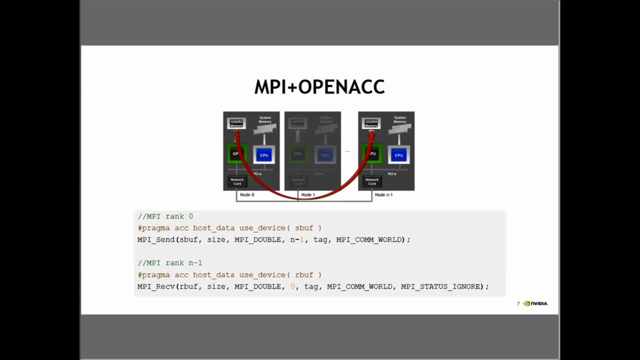 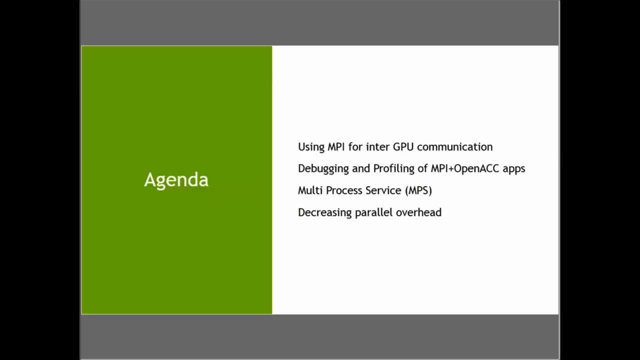 and therefore you would be communicating data if you send the device at the host representation. Okay, What's the agenda for today after this short introduction? So first I want to explain by example how to use MPI for inter-GPU communication. 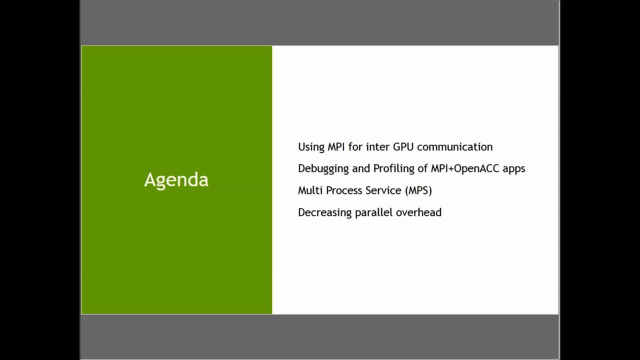 Including a very brief introduction to MPI. Then I will talk a little bit about how to debug and profile MPI plus OpenACC applications, Touch on the multi-process service and how it can help to improve speed up when porting legacy MPI applications to OpenACC. 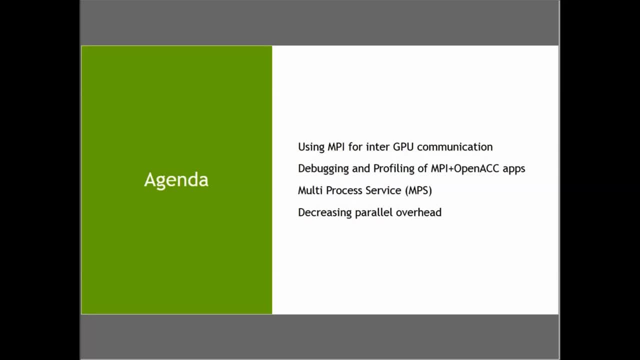 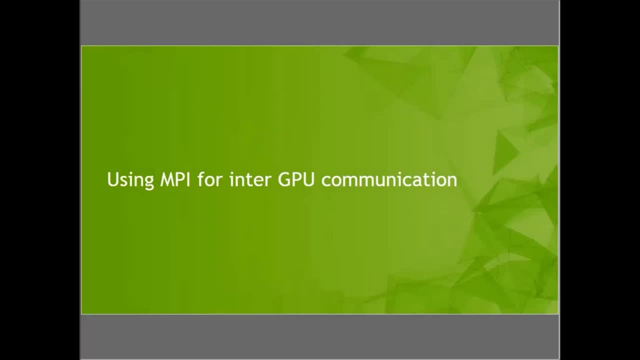 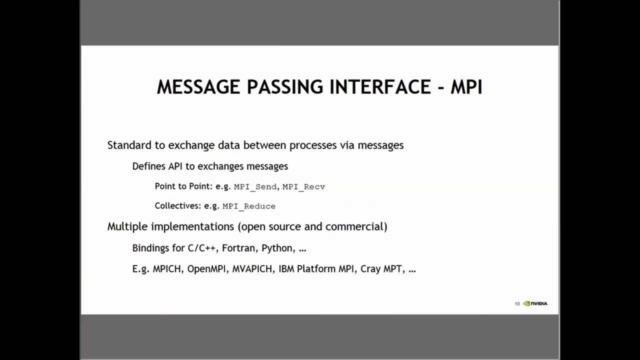 And, finally, how you can decrease parallel overhead and improve the scalability of your program. Okay, Let's start with using MPI for inter-GPU communication. First, what is MPI? It stands for the message passing interface and this is standard to exchange data between processes via messages. 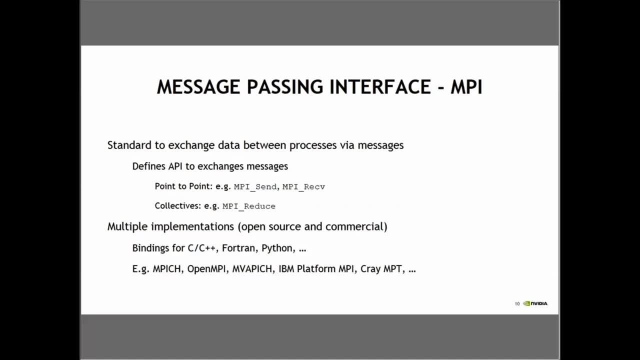 It defines an API to exchange messages where we have different classes point to point, For example, MPI send, MPI receive, or combined MPI send-receive operations, or also non-blocking versions, MPI I send, I receive, And besides that also collective operations like MPI reduce or reduce, and so on. 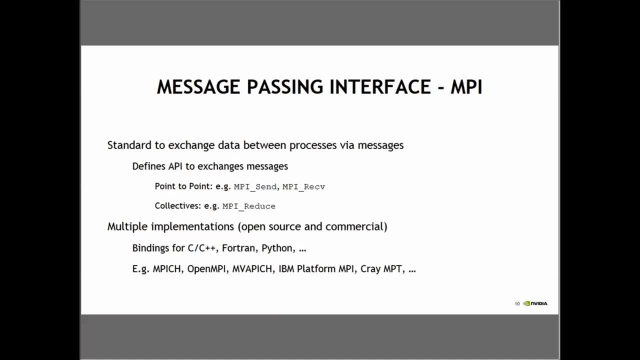 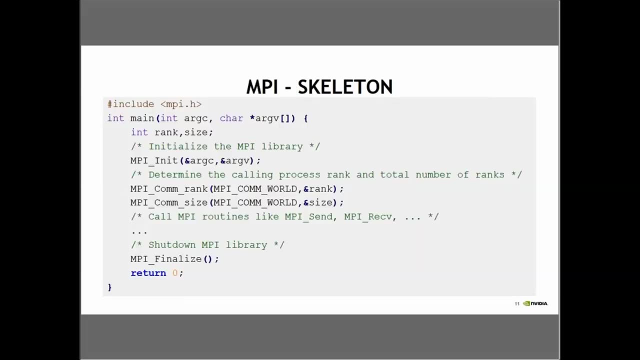 There exist multiple implementations, both open source and commercial, with bindings for C, C++, Fortran, Python and so on. Just to name a few examples: OpenMPI, MVAPitch and MPitch. So how does an MPI code look like? 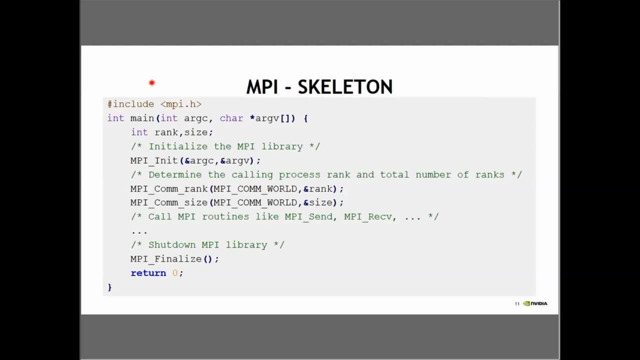 I'll give a very brief skeleton. You first have to, of course, include the header defining the MPI API mpih. Then you have to initialize. Before you can call any other routine from the MPI routine, you have to initialize the MPI library by calling MPI init. 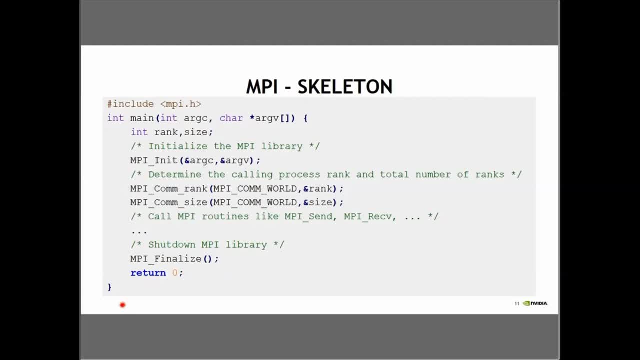 And corresponding to that, at the end of the program you should clean up after yourself and call MPI finalize. Between that, you can do this, You can do any call all MPI routines to coordinate the work of all the participating processes. I want to highlight here two things that are usually called first. 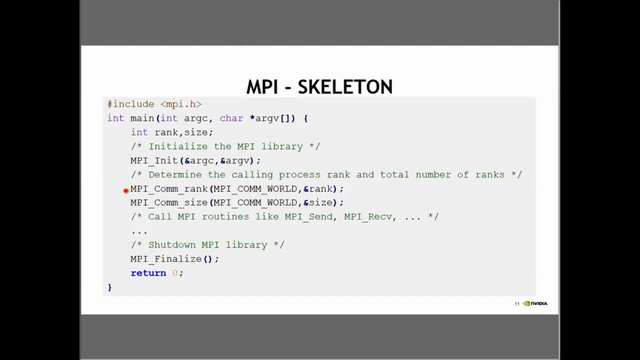 because they are needed to identify the process in the set of processes participating in the run. So the first one is MPIComRank, which returns an ID from zero till size minus one to the calling process so that it knows its unique ID within the set of processes and can coordinate any communication. 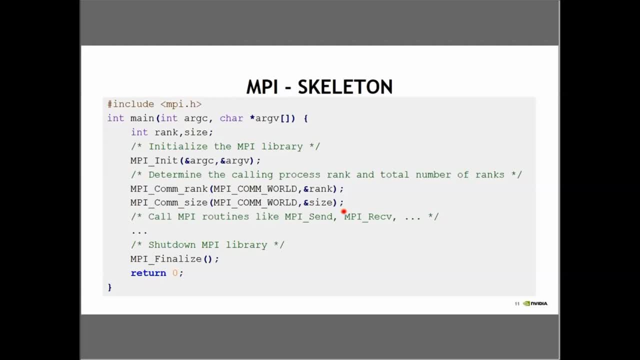 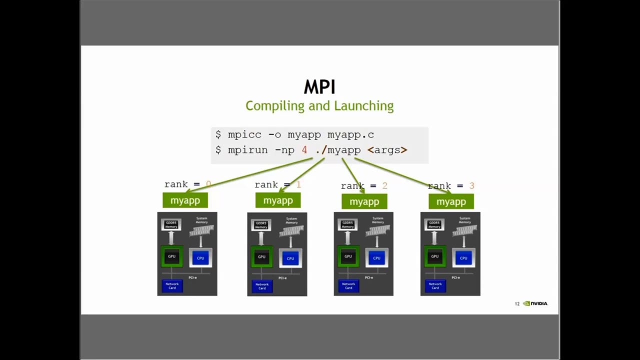 And the second one is MPIComSize, which returns how many processes are participating. Okay, I will explain by example how these values can be used later. Let's first take a look how this one is compiled and launched. So compiling is just done like with regular compilers, just that you need to set include paths and library paths correctly. 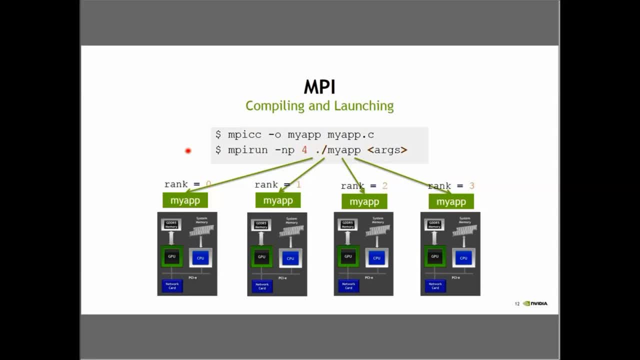 And to ensure that usually MPIs- MPI implementation- come with a compiler wrapper which, in case of C, is called MPICC. So you just use MPICC instead of your regular compiler and compile your program. Next thing is you need to launch multiple instances of MPI. 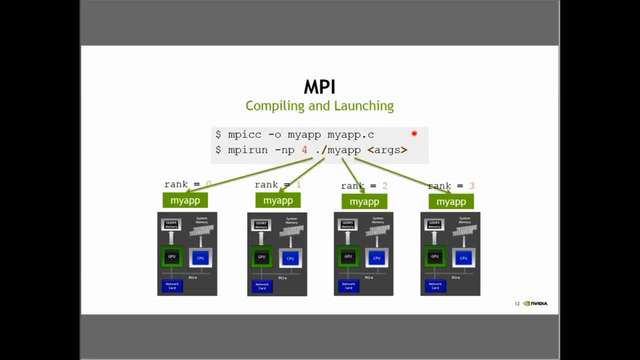 So that you have actually many instances that can work in parallel. For that MPI implementations provide so-called launchers, which are not always named the same. Often they are named MPIRun or MPIXec. On Serum systems, you sometimes have to call Srun. 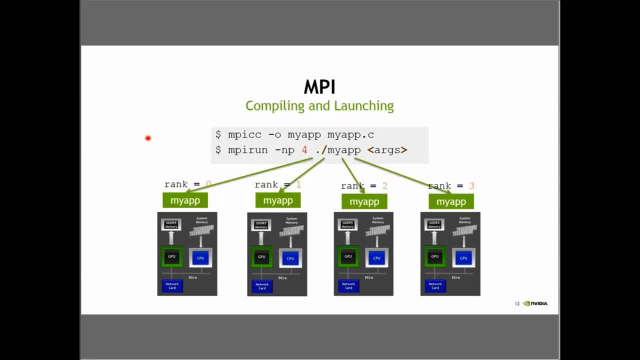 On Cray systems, you need APrun. But they all usually have sometimes different names, So we named one important, the most important argument, besides others which are for fine-tuning process placement and are not covered in this talk- It's the dash NP argument which says how many instances I want to launch. 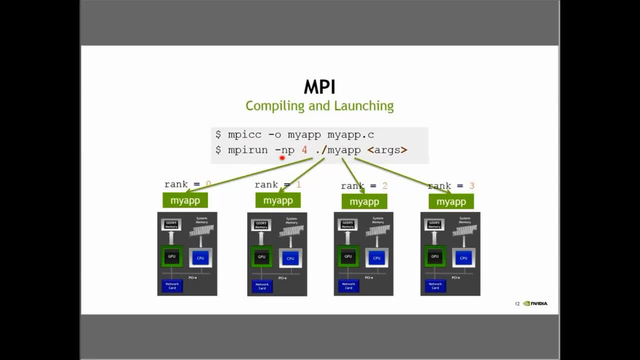 So you just prefix your application with MPIRun, dash NP, in this case four, to launch four instances, and then your application and arguments, And that will spawn four instances of your application to four nodes of your cluster, To one node with four GPUs of your cluster. 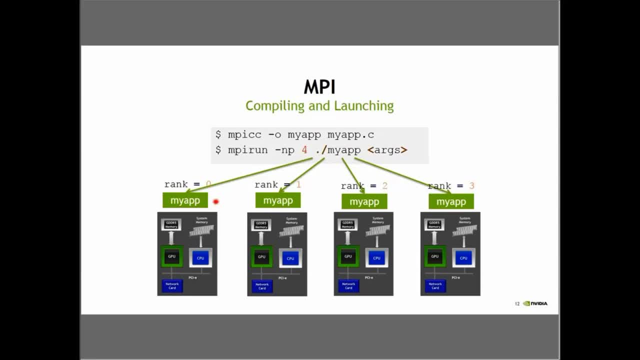 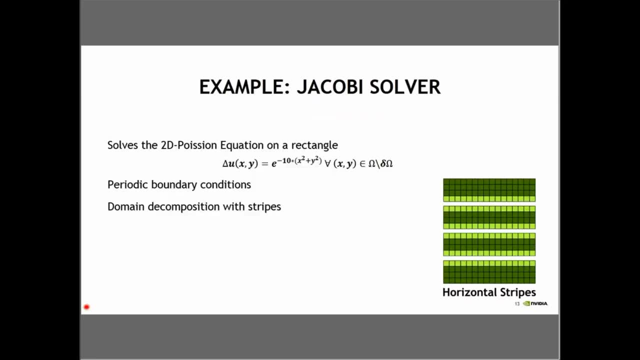 And sets the rank to zero for the first, one to one for the second, and so on. Okay, So how does an MPI application look like? Let's take a look at an example: A Jacobi solver for the 2D Poisson equation on a rectangle with a given right-hand side which has periodic boundary conditions. 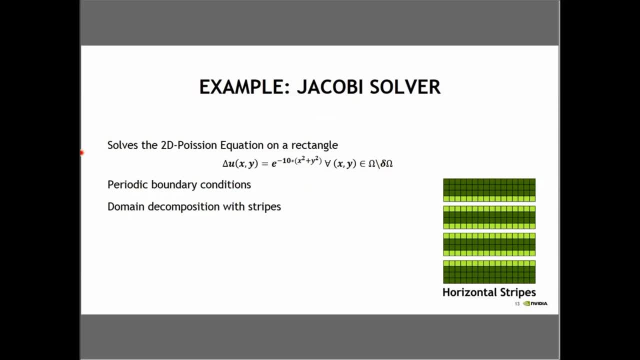 And to distribute the work across multiple GPUs. we do a domain decomposition with stripes. So, as you can see, on the right we're assigning, we're dividing our domain in four smaller subdomains of the same size and assign each domain to one GPU. 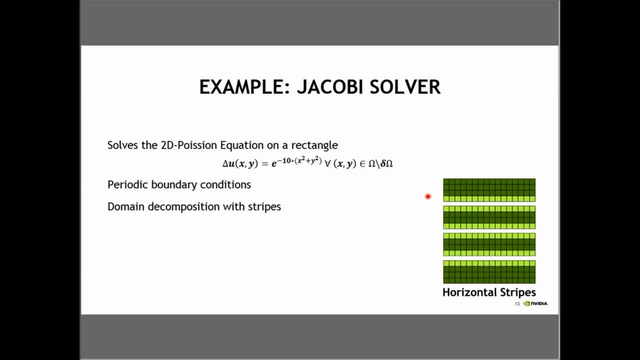 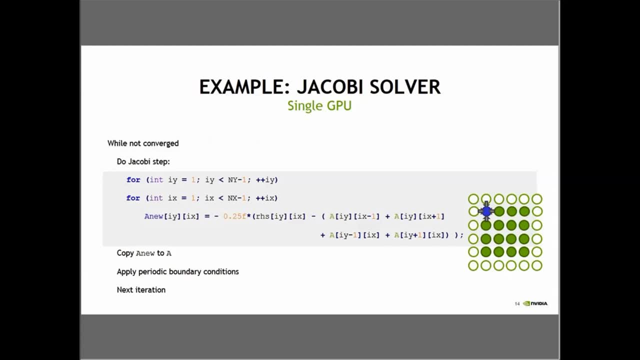 And then exchange data between them via halo regions, which are shown in light green. Okay, Let's first take a look at the single GPU, Jacobi solver, so that you're reminded or get an idea of what it does. So it executes a while loop until it's not converged. 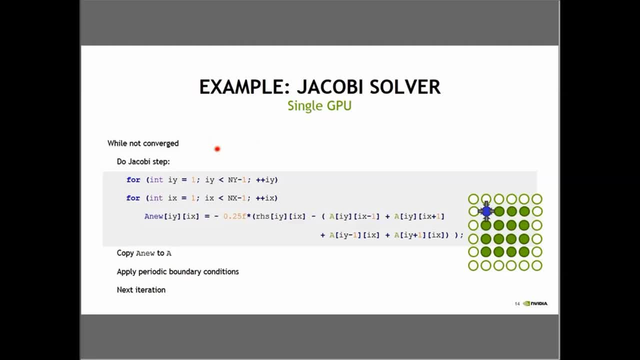 And in each iteration of the while loop it executes one Jacobi step which iterates over all interior points of the domain And essentially calculates an average of the four neighboring points, writing to the variable anew. After that step anew is copied to a. 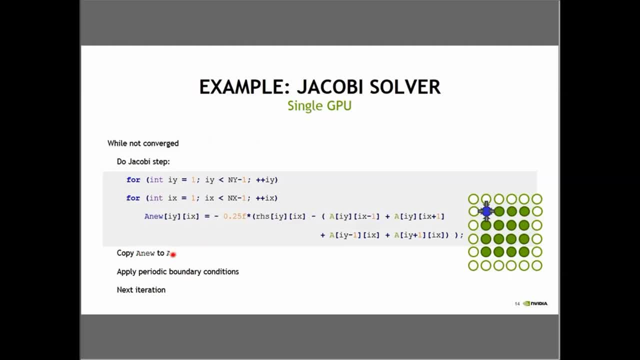 So that these two representations are swept and the next and anew can be used for the same purpose in the next iteration. And then the periodic boundary conditions are applied, which is essentially a copy of the last modified row to the top boundary, a copy of the first modified row to the bottom boundary, a copy of the first interior column to the right boundary. 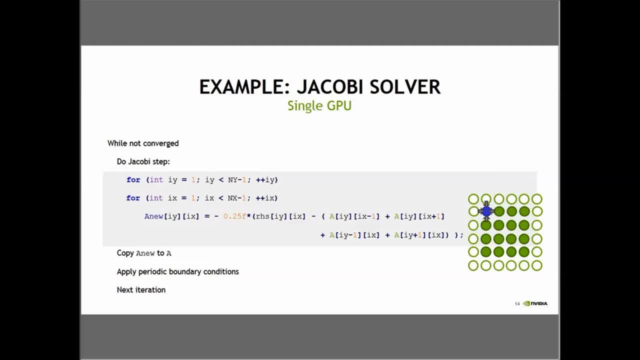 and a copy of the last interior column to the left boundary, And then the next iteration is done, And then the next iteration is started. Okay, How can we do that with multiple GPUs? As I said, we are dividing our domain in multiple stripes. 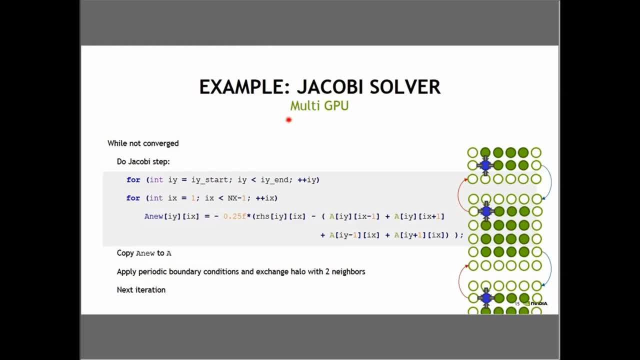 And every GPU is then only working on the stripe assigned to it. In this case, the GPU currently looking in this case is starting at the row IY- start, and computes till the row IY- end, Because each GPU only works on one GPU. 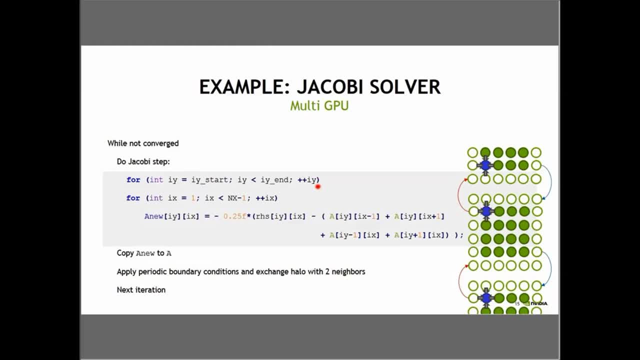 Okay, Each GPU only works on a subset. We now need, after copying A to anew, we need to exchange data so that information can propagate over the whole domain, And for that each rank leads the sensor last row. it has modified to the top halo of the bottom boundary. 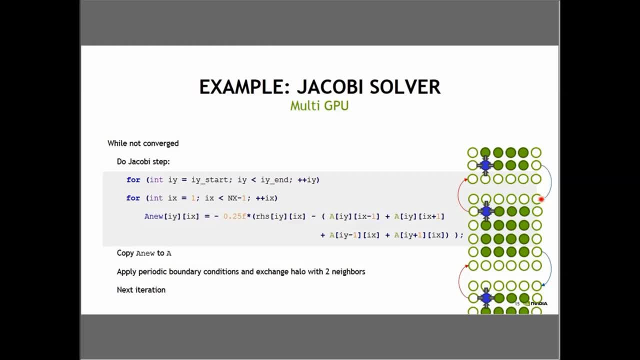 to the top halo of the bottom boundary And the top in a row it has modified to the bottom halo of the top neighbor. So these halo regions, thinking about each rank as a single GPU, these halo regions can be treated essentially as the boundaries. 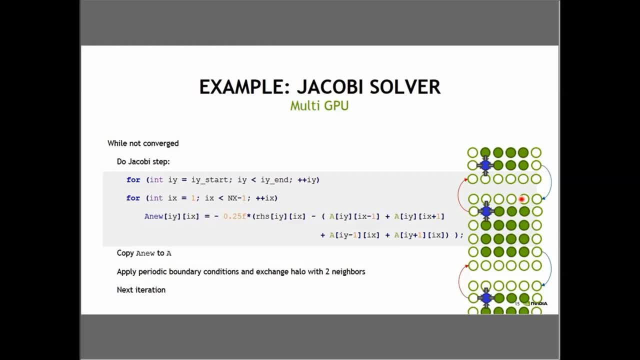 And the boundaries of the global domain are the real boundaries, And the boundaries in the inner domain are to exchange data between the GPUs and are called halos. Okay, How does this communication of halo values work with MPI? So let's take a look. 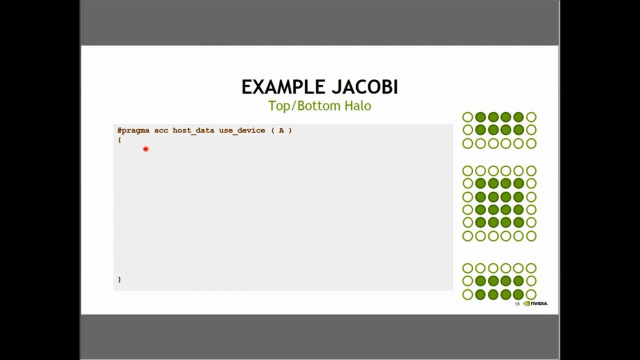 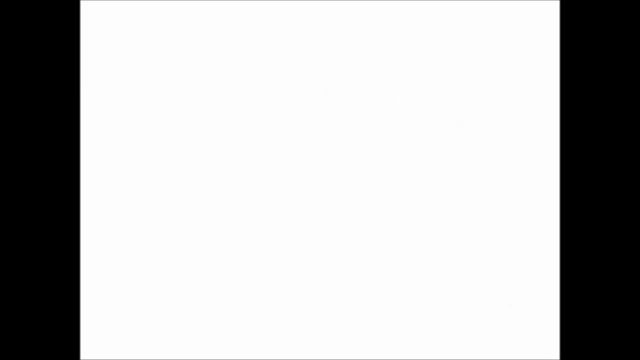 First, as I already mentioned, it's important that you, because we are working, we are solving, we are executing the solver completely on the GPU, So we are modifying the device representation of our field A. So it's important to use the pragma ACC host data use device so that always the device representation and not the host representation with data pass to MPI calls. 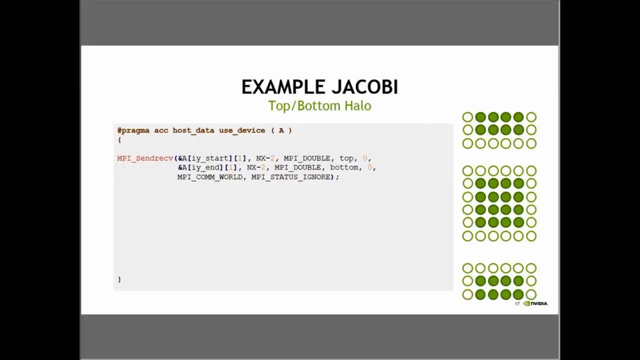 And then, in the first step, we call MPI, send, receive, which is a combined send and receive, And send the first modified row to our top neighbor And receive to our bottom halo from our bottom neighbor. The second step: we receive our top halo from our top neighbor and send the last modified row to our bottom neighbor. 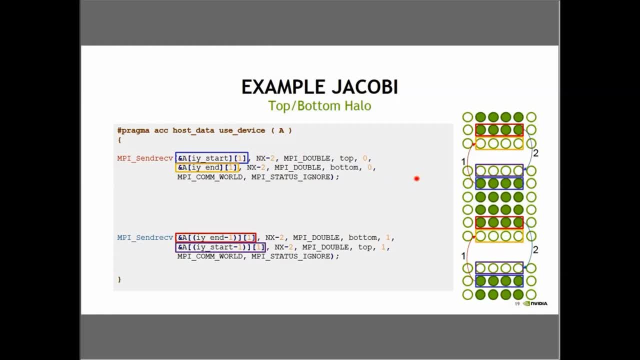 Okay, Okay, Okay, Okay, Okay Okay, the top neighbor of rank zero being the last rank and the bottom neighbor of the last rank being rank zero, this will also automatically handle the periodic boundary conditions. Okay, that essentially explains how you can. 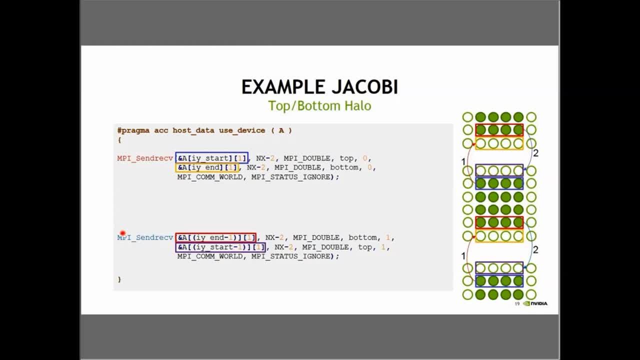 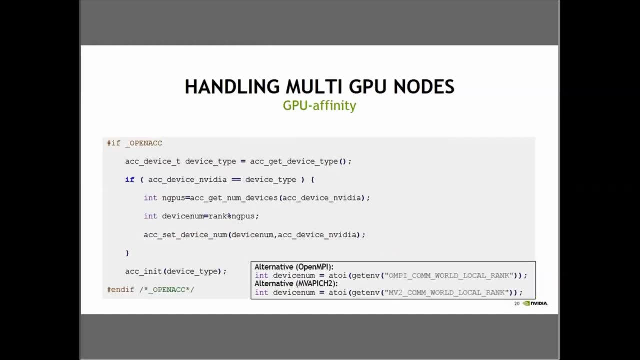 communicate data between GPUs. So you know how to compile an MPI program, how to start it, how to exchange data between GPUs. One thing you need to know in addition to that is how to handle GPU affinity, because if you're running on multiple 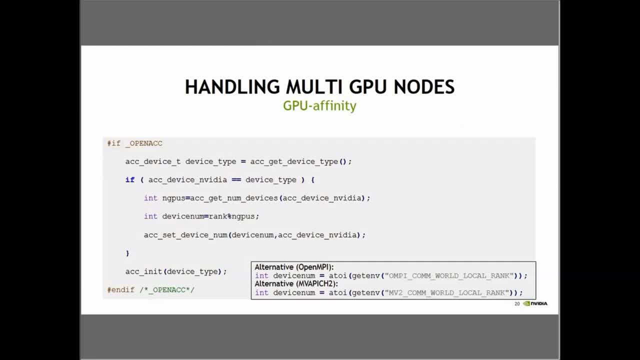 on nodes with multiple GPUs. you have multiple MPI ranks running on each node and they need to coordinate which MPI rank should use which GPUs, because otherwise they would just all use GPU zero and you would oversubscribe GPU zero and you'd leave GPU one, two and three idle. 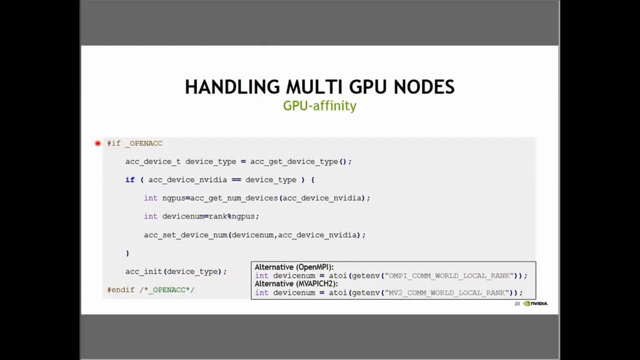 So to do this with OpenACC. I've protected that with preprocessor macros so that you still remain have a program that works without OpenACC. You query in case you're using an NVIDIA device with separate memory and not, for example, the multi-core targets also supported. 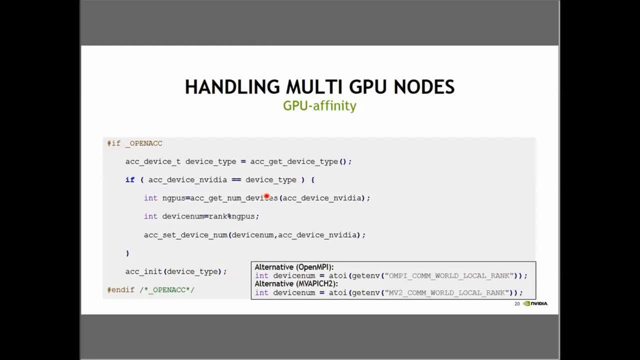 by the OpenACC implementation by PGI. you query how many GPUs you have in a node, and then a simple assumption would be that you rely on ranks to be consecutively placed on each node, So that rank zero if you start four ranks per node. 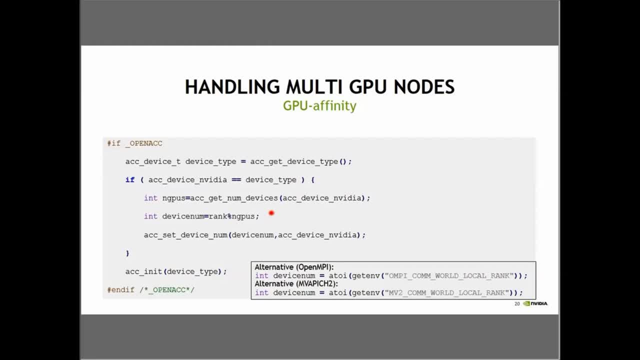 that rank zero, one, two and three are all placed on the same node and rank four, five, six and seven are placed on the next, next node, and so on. And then you can use a model operation of your rank by the number of GPUs to select the device you want to use. 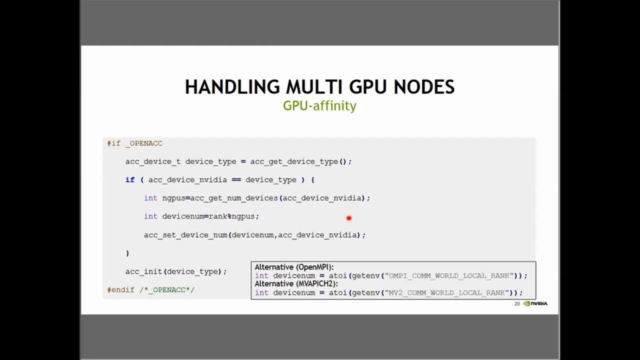 by calling ACC to set device number on that device number. An alternative to that would be to use environment variables provided by the MPI launcher. For example, the launch of OpenMPI sets OMPICOMWORLDLOCALRANK, which this the ID of your. 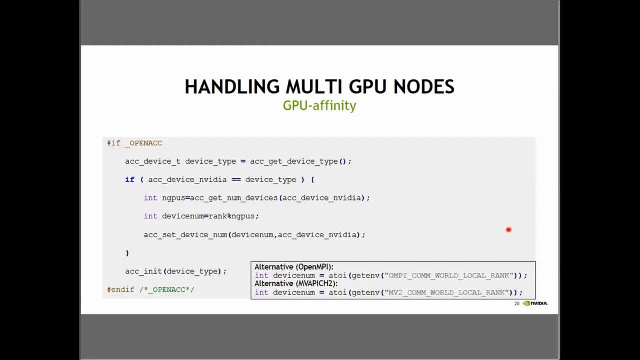 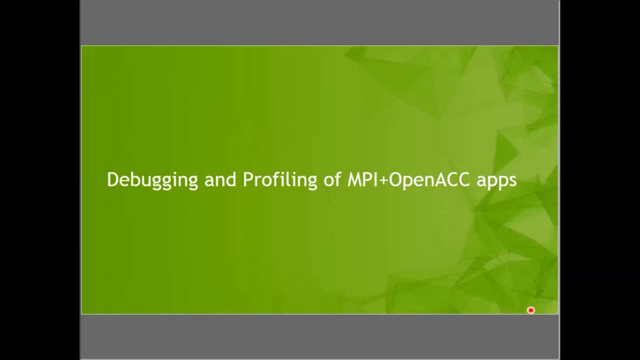 your MPI rank just within the node you're running on. So you could also just call A2I, GETENV, OMPICOMWORLDLOCALRANK to get the device number. Okay, I see there are some questions. Let me try to answer them now. 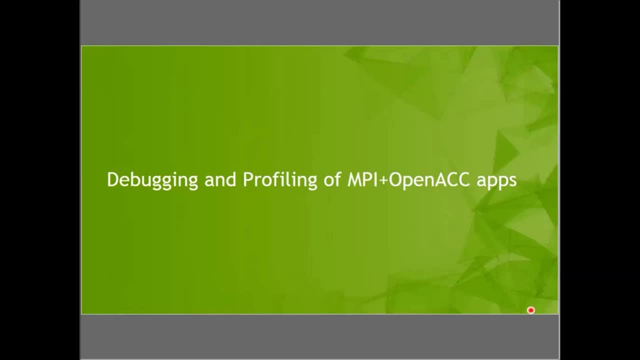 before jumping to the next question. So the first question is: can we use MPI and PGI FORTRAN along with OpenACC? Yes, of course I'm presenting all the examples in C- C++ on the slides, but the homework is available in C, C++ and FORTRAN. 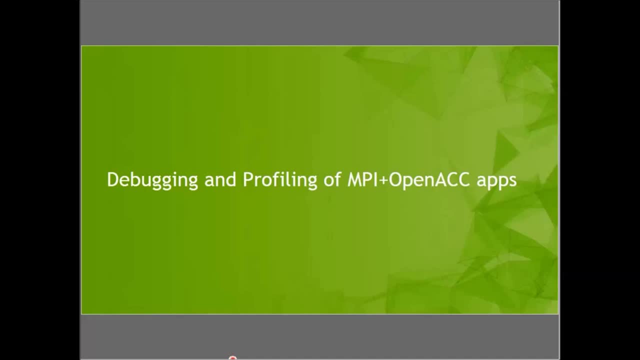 And the concept is exactly the same, Just the syntax would be slightly different. Yeah, just what is needed with FORTRAN compared to OpenACC. Second question is: I'm familiar with MPI for multiple processor and processors and threading for multi-core processors, And what are my thoughts on this? 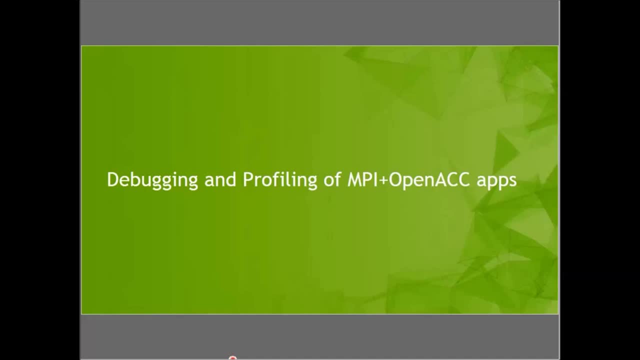 Yeah, that's actually when. When you compare MPI plus OpenMP, parallel program programming-wise it's very similar to programming MPI plus OpenACC. The only essential is start. in case of MPI plus OpenMP, you would start one MPI ring per CPU socket. 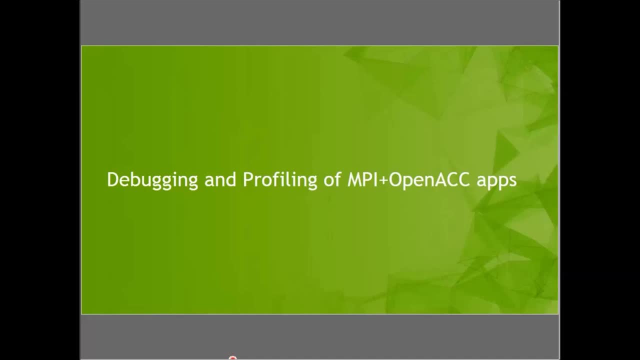 and then use as many open MP threads as the CPU socket has cores. In case of MPI plus OpenACC, you would start one MPI rank per OpenACC device and use OpenACC for the parallelization within the OpenACC device. Next question is: can we use MPI send, receive? 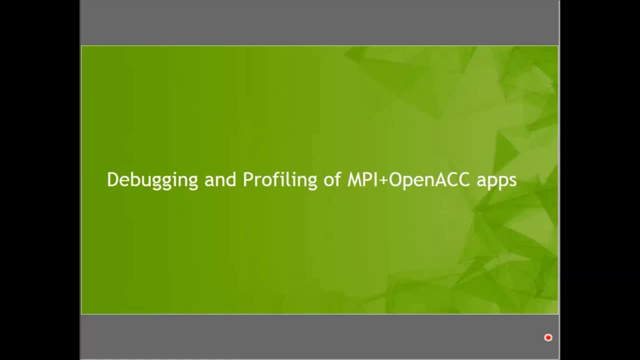 inside compute regions? No, that's not possible. MPI is the host side API and can only be called from host code. So you can directly call send from and to GPU buffers, but the communication is handled by the CPU. And another question before I continue. 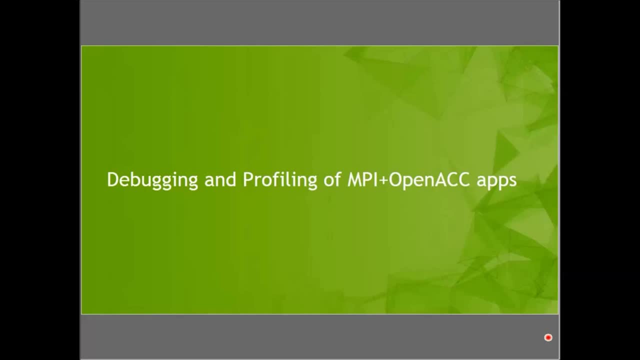 with the next session is: if an MPI node has multiple cores and a single GPU, should we use OpenMP for the cores and OpenACC for the GPU? You can, That's a very good question. You can do that If it makes sense. really depends on your problem. 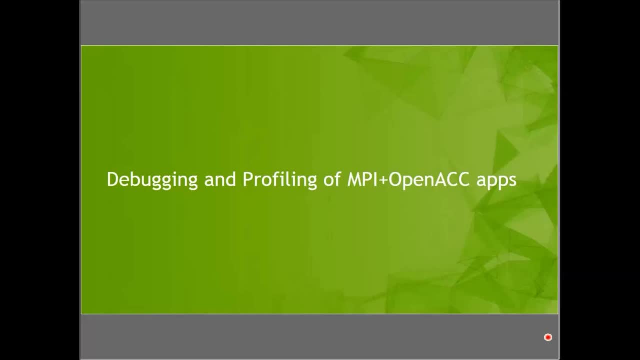 The thing is that usually the performance of the CPU and the GPU is usually quite different. So you need to take care of load balancing And usually taking care of that adds some overhead And if it pays off at a net effect really depends on your application. 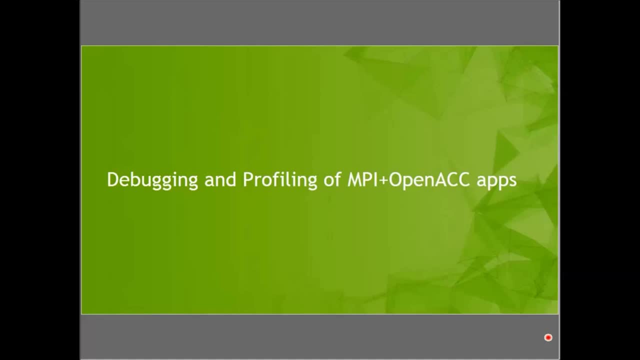 Oh yeah, there's one more question coming in which I can answer now before continuing. If all GPUs are installed on one computer, do we need to use MPI? No, you don't need to use MPI. You could also, for example, use OpenMP. 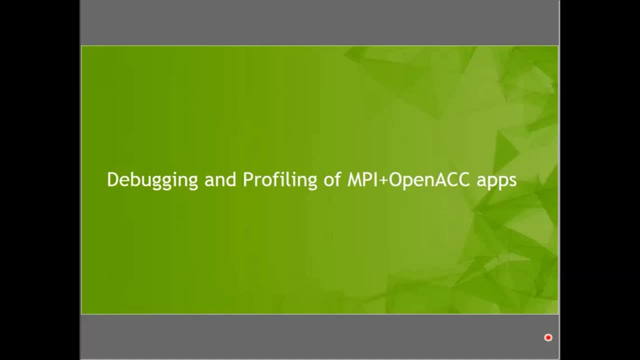 to start one CPU thread per GPU, Or you can just call ACC set device and switch the view and control all GPUs. OK, So you can use both GPUs from a single device. However, you can use MPI also within the node And so it works within the node and allows. 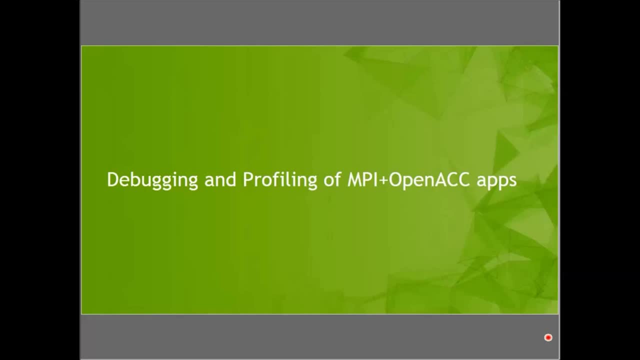 you to scale beyond the cluster And, furthermore, compared to the other two approaches, it has the advantage that you can transfer data directly between GPU buffers with GPU peer-to-peer. This functionality is currently not available with the other approaches. There was a follow-up question on the OpenMP and OpenACC. 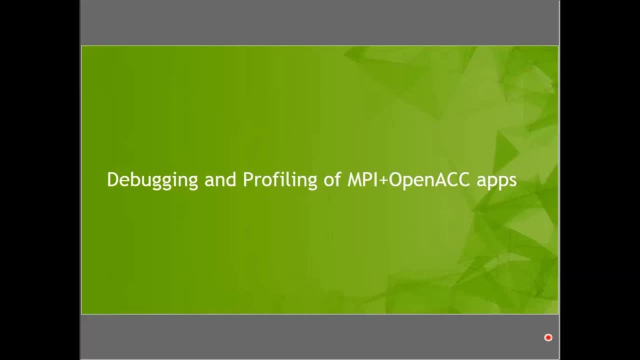 question for the course. Currently it's not possible to build set binaries with OpenACC for multi-core and GPU. So each MPI rank- and even if each MPI rank would need to decide if it wants to use an OpenMP, an OpenMP- 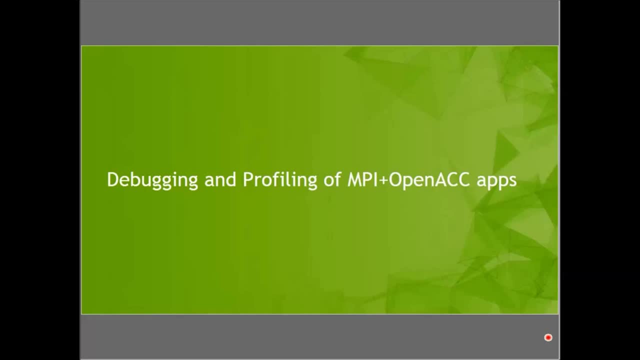 a GPU or the multi-core And therefore you could use that with a FET binary by just launching two MPI ranks per node and then deciding which one uses which target, But still you have the load balancing problem. There are more questions coming in. 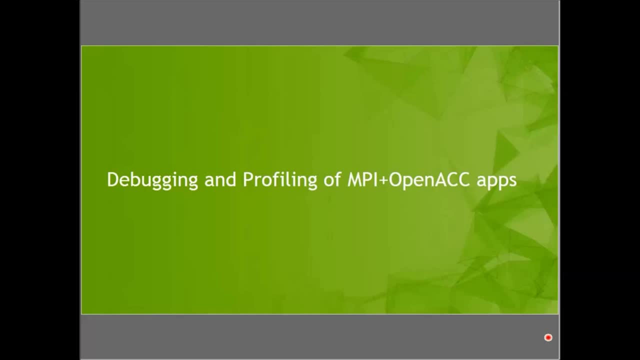 And so I think we can still answer them now. How do we know if we can use CUDA, GPU-aware MPI, and if there's a runtime check or a compile time check? Unfortunately, there's nothing. no standard way. However, OpenMPI defines a macro and a function. 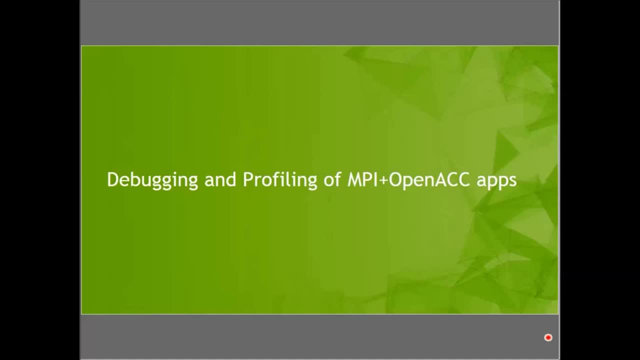 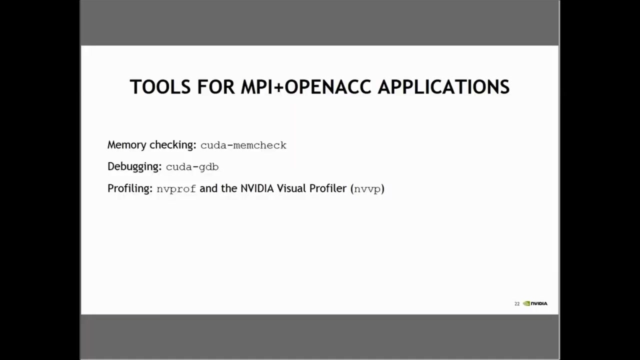 you can call during And you can use that runtime to check for CUDA awareness. For that you have to include the MPI X header. OK, let me continue with debugging and profiling for MPI and OpenACC applications. So I want to introduce three tools for. 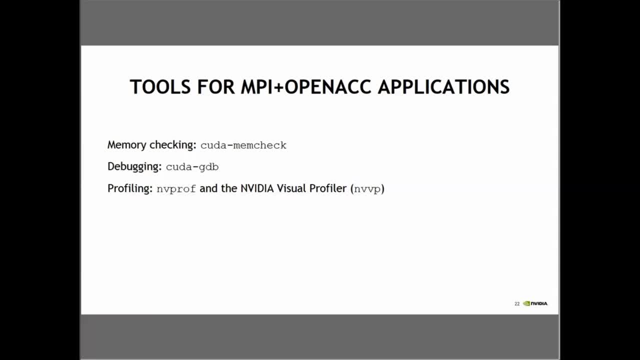 which are relevant for MPI plus OpenACC development. One is CUDA MPI, The other is CUDA MemCheck, which is a memory correctness and checking tool like VALGRAND. Then you can use the GPU debugger CUDA GDB for OpenACC programs, where it compiles with debug information. 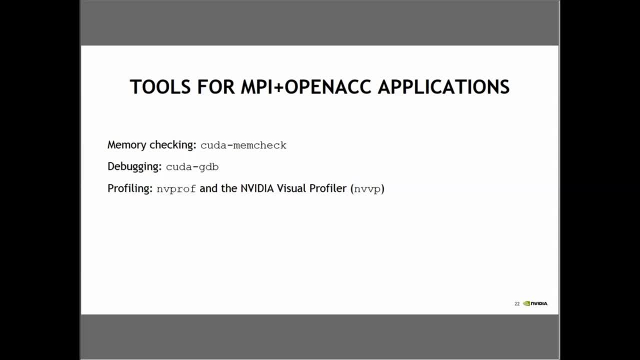 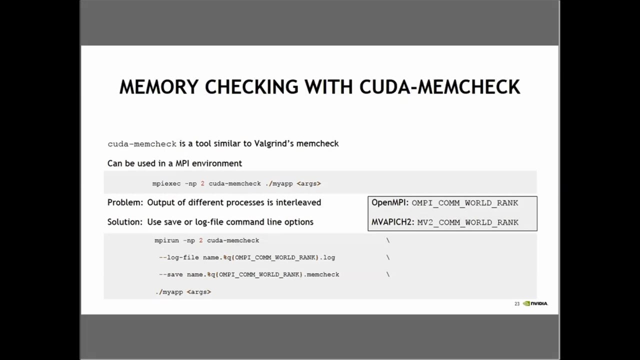 And furthermore, you can use NVPROF or PGPROF and the visual profiler to profile MPI plus OpenACC applications. OK, let me start with memory checking with CUDA MemCheck. So I'm going to start with memory checking. So yeah, CUDA MemCheck is a tool suite very similar. 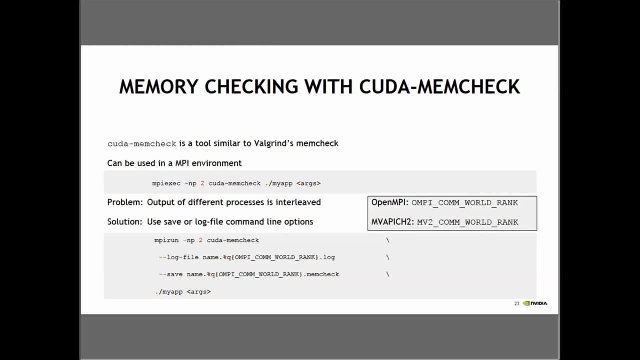 to VALGRAND's MemCheck And it can be used in an MPI environment. just straightforward: Just launch one CUDA MemCheck instance per MPI rank with your application. So use MPI exec as a launcher for CUDA MemCheck, which is used as a launcher for your application. 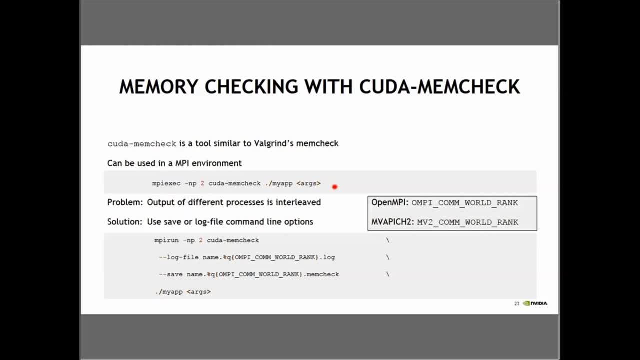 This works but usually produces quite some unreadable output, because CUDA MemCheck doesn't know about MPI, So every rank writes to a standard out And therefore the output of all processes is interleaved, which is hard to read. There's a solution to that by using environment variables. 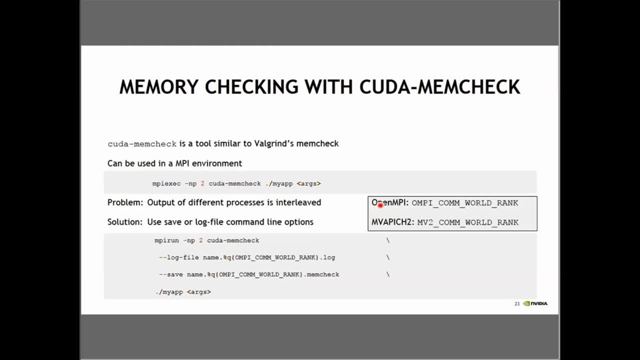 provided by the MPI launchers, which is in case of OpenMPI, oMPIcomworldrank And in case of MVAPitch2, MV2.comworldrank. Another MPI might define a different, probably different, finds, a different variable. 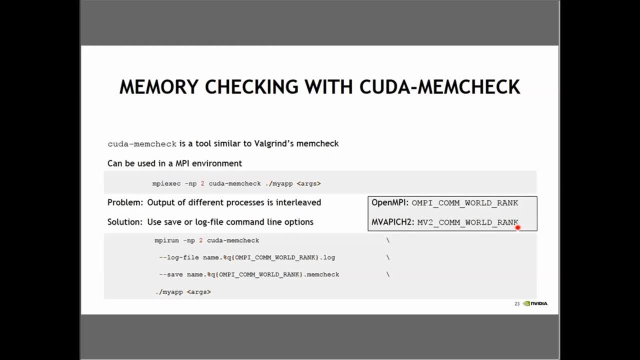 For example, I've seen PMI rank being set. This environment variable contains is set differently for each instance and matches the rank in MPIcomworld, So you can use that to pipe the output of CUDA MemCheck to a named file. In case of CUDA MemCheck you have two options. 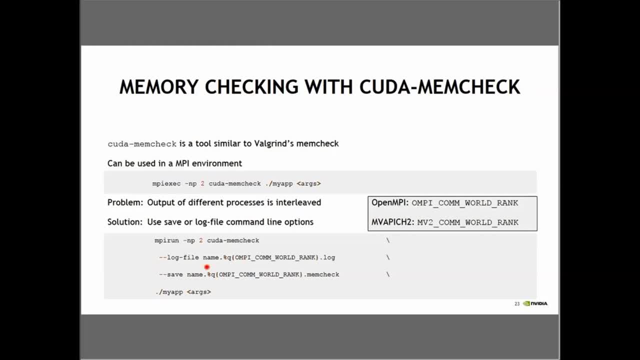 dash, dash log file, which saves the textual output, and save, which saves the binary output which you can later read in with CUDA, MemCheck, And then percentage queue, curly brackets and the environment variable will replace at runtime this expression with the value of the environment variable. 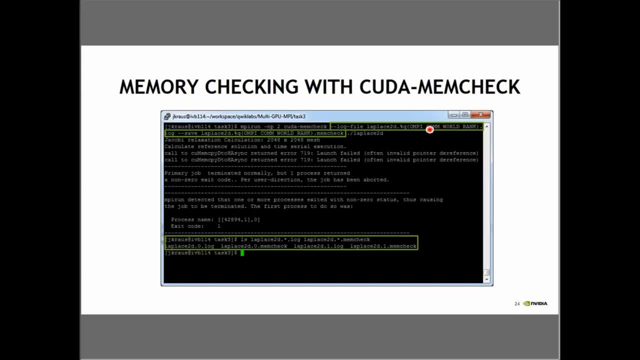 So, to give a short example, if you pass these variables, it will produce a log file for each rank. So I've started with two ranks. So I get a log file for 0, a binary file for 0, a log file for 1, and a binary file for 1.. 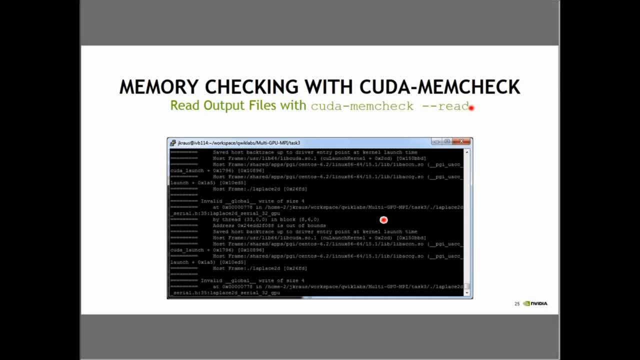 And the binary files I can read in with CUDA MemCheck read And then I get just the regular CUDA MemCheck output identifying the issue in my MPI plus OpenACC program. This is helpful. It's able to identify a lot of errors And hopefully you don't need to dig further. 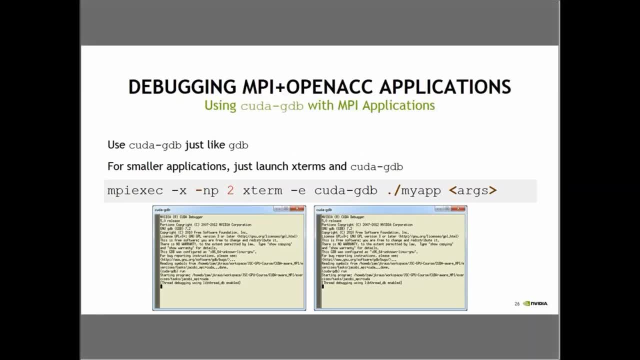 But if you need to, you can also use CUDA GDB with MPI permutations, just like you probably know how to use GDB in an MPI environment, For example, for small applications. you can just start at xterm with a CUDA GDB. 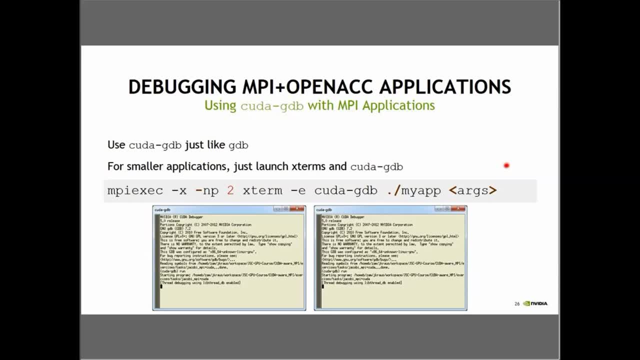 instance, for every rank. This is, of course, not scalable because if you imagine, with 256 MPIs, Having 256 MPI ranks, having to manage 256 xterm and CUDA GDB instances is probably not very good. So there are a few other options. 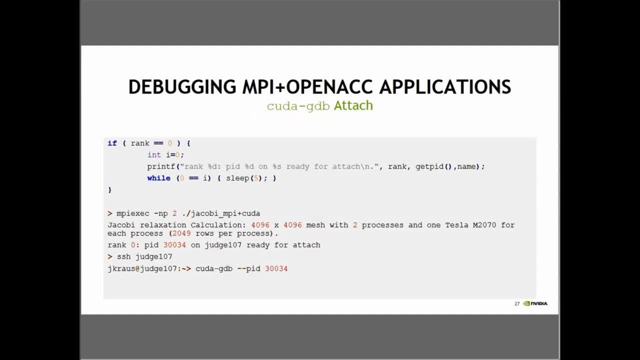 First one is that you can attach to a running process So you can do it programmatically by just inserting an infinite loop where you need to change a variable in the debugger and print the PID, the host name and the rank just before entering an infinite loop, so that you 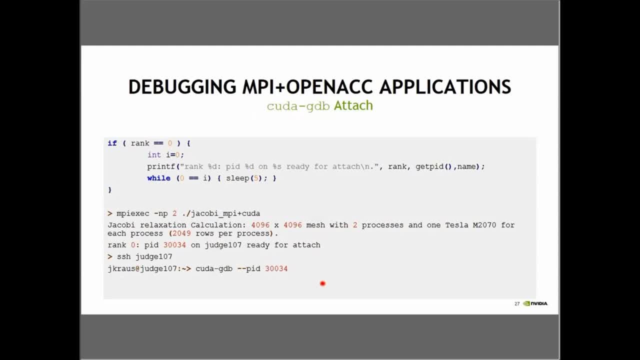 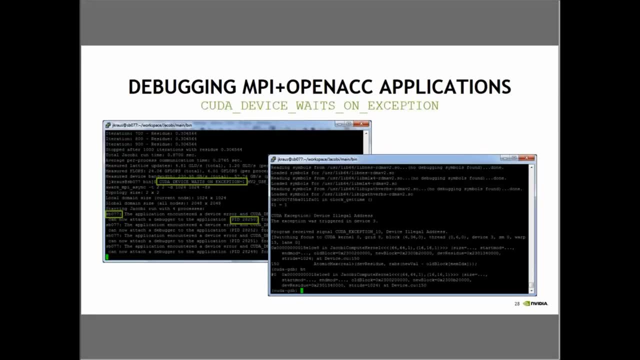 can then just use CUDA GDB to attach to the process. There are two more environment variables I want to mention. One is CUDA device weights on exception. If that's set to 1, a process will if it hits, for example. 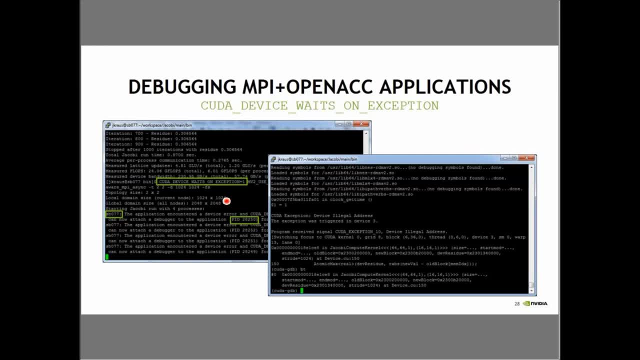 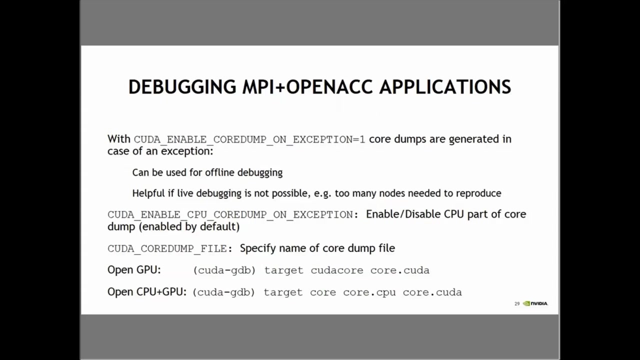 out of bounds memory exceptions. it will not crash. It will hold and print a message containing the host name and the PID. You can use that to attach to it and inspect the state and hopefully identify the issue of your application. Furthermore, you can generate core dumps. 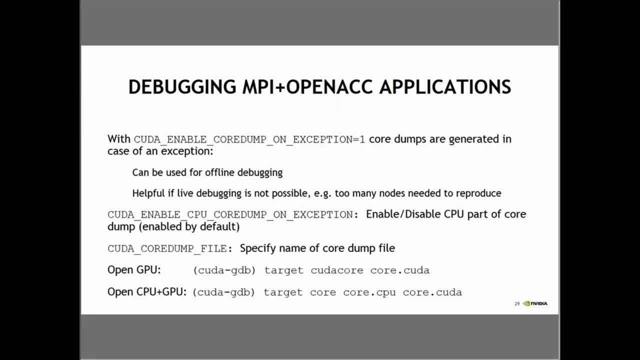 If you're set CUDA animal core dump on exception to 1, and you can selectively decide to also create, I believe, a core dump on exception, It will always contain a GPU core dump and you can selectively decide if it should also contain a CPU core dump, which might make sense. 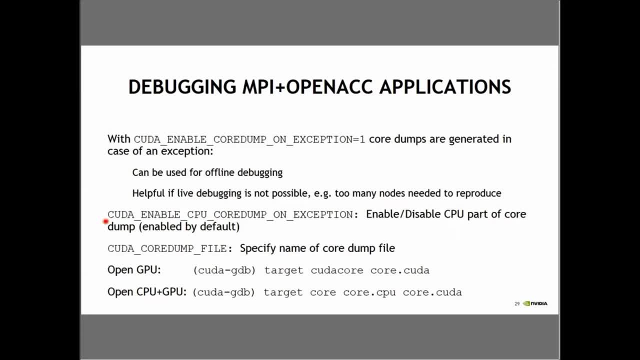 to throw that off to save some space. The CPU core dump feature can be set with CUDA animal CPU core dump on exception And these core dumps then can be used for offline debugging and are helpful if you can't do live debugging because you need too many nodes or you can only submit jobs via a batch system. 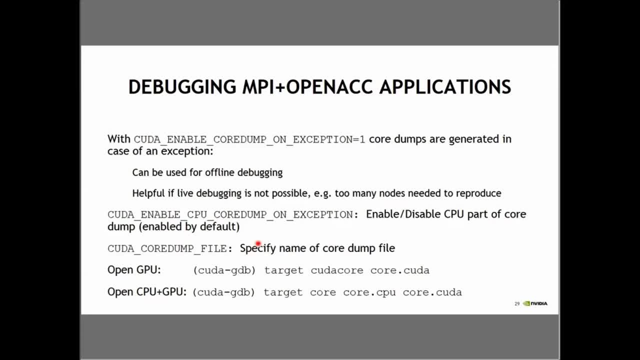 or so on. You can also define the name of the core dump file and then in CUDA GDB you can open them with target CUDA core to open just the GPU core dump, or with target core and then the core file of the CPU and the GPU. 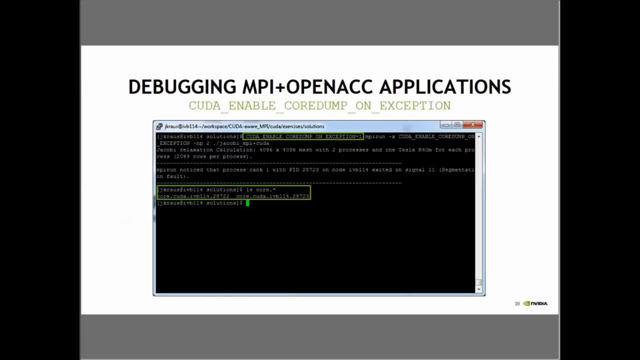 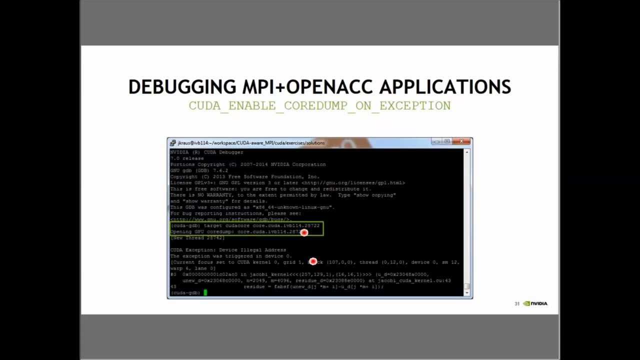 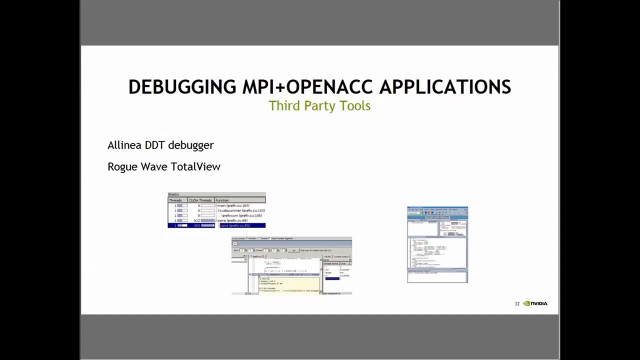 to open both of them. To give an example of that: if you set that you get the two files and can open them and then expect inspect the state, You can identify the state of your program to identify the error. Besides this, there are also third party tools. 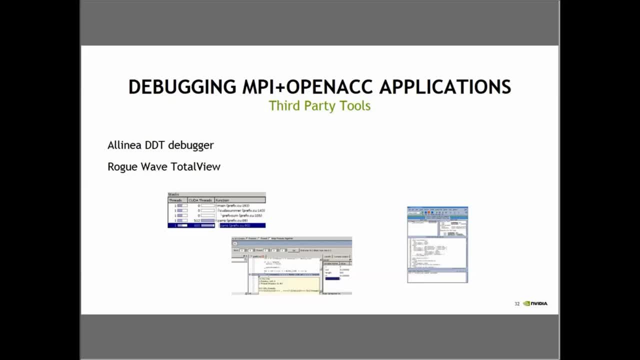 with scalable debuggers which you probably know from other MPI experience. The Alinea DDT debugger is GPU aware and the ROOT wave total view debugger is also GPU and OpenACC aware. OK, Now you know how to build, to write an MPI plus OpenACC program and you know how to debug it, so you probably want. 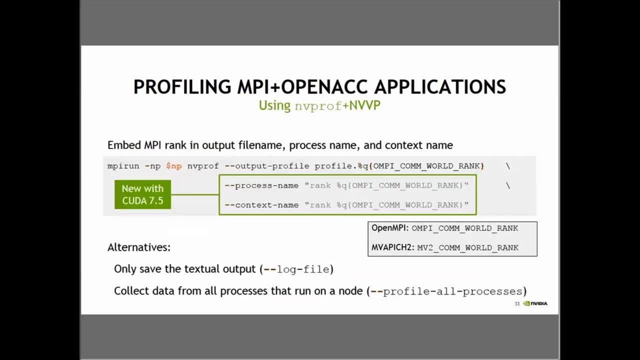 to improve performance. So let's look into profiling MPI plus OpenACC applications. You can use the NVPROF and NVVP for that And, just like with CUDA GDB, you just start MPI run. use MPI run as a launcher for NVPROF. 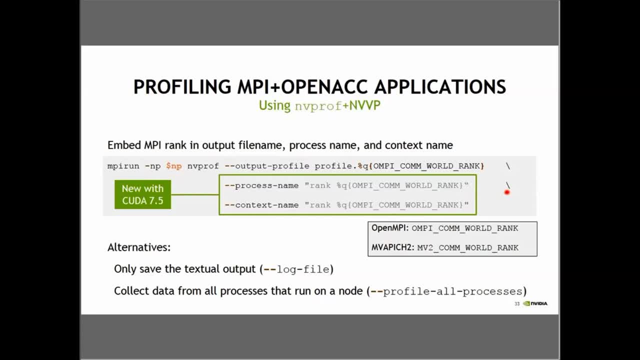 which is used as a launcher for your application. So again, here is that output would be interleaved. but you can use the same trick by using the environment value of OMPI, com, world rank for OpenMPI and so on for others to pass the output. 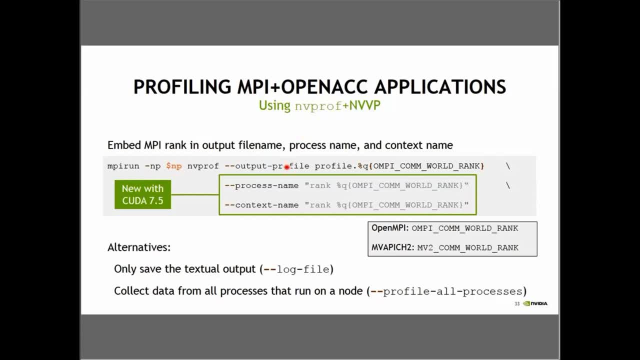 to create one output file for each rank with the output profile option. With CUDA 7.5, we introduced something more: that you can also name the process and the context name shown in NVVP with the options dash, dash, process name, and then you pass in. 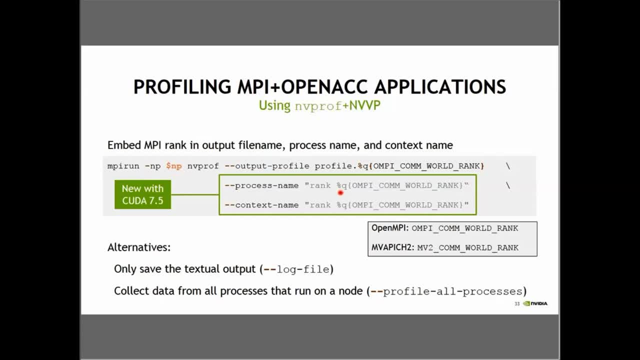 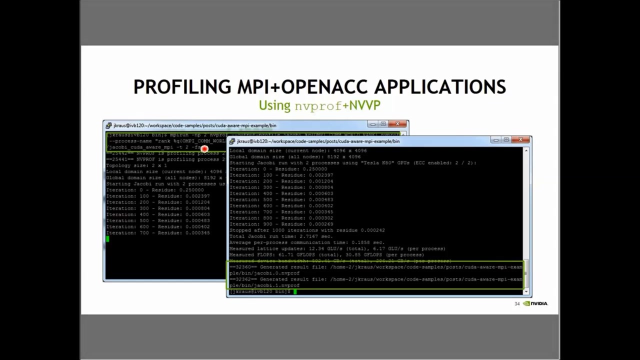 the string where the environment variable with a percentage Q is also replaced with the rank and the where it is created. for Alternatives, you could also profile all processes on the node with the profile all processes option or only save the text. Okay, doing that, we'll create one MPI and again starting with two MPI ranks, and it will 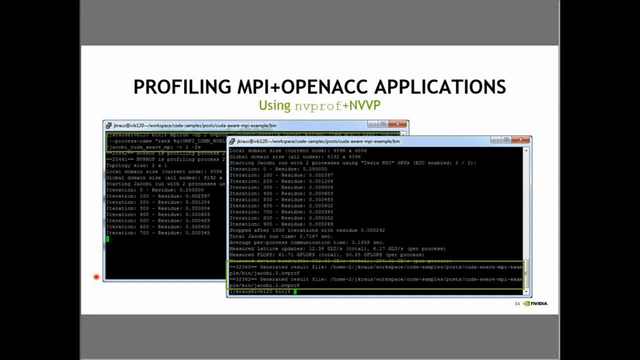 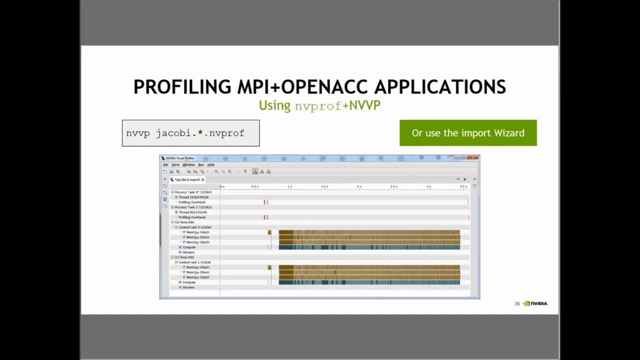 create two files, one for each MPI rank named with zero, which can be imported into NVVP with the import wizard selecting the multiple processes view And then you'll see process MPI rank zero. process MPI rank one. the context rank zero running on a K80, context rank one coming on a K80 and, I think, work in parallel. and 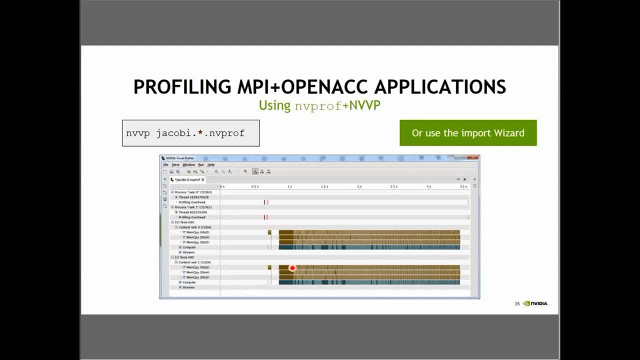 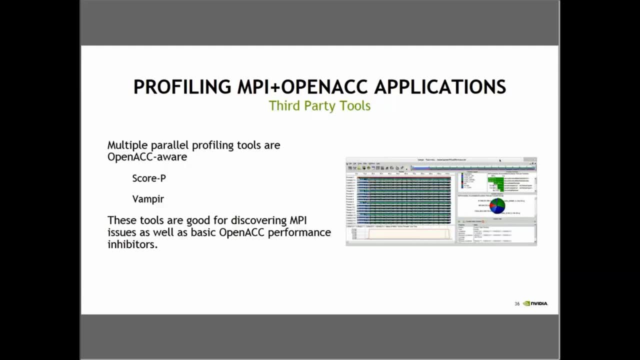 you can see if there are node balancing issues and how the communication works, As with the debugging. there are also third party tools which, especially with regard to MPI profiling, are far more powerful, And also I want to highlight here Scopee, which is a tracing framework, and Vampir, which allows 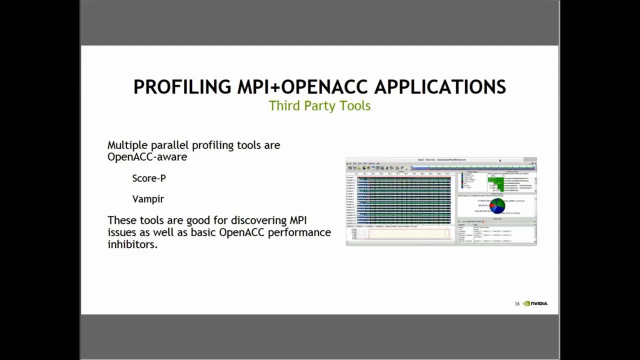 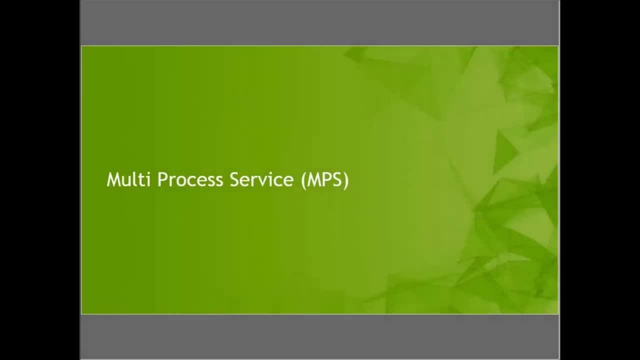 to view these traces and the communication patterns and so on. Okay for starting going to the next session, let's take a look if there are some questions. Okay, I think there are no unanswered questions, so let's continue with the multiprocessor. 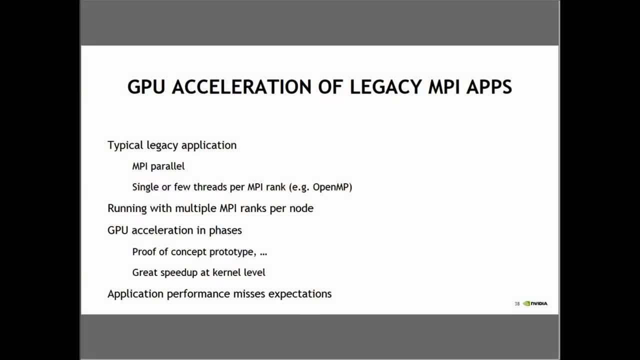 The multiprocessor is interesting for GPU acceleration of legacy MPI apps, So typically legacy application. You might be working on this, probably MPI panel, and might use a single or a few threats per MPI rank, for example with OpenMP, And so usually you would run with multiple MPI ranks per node and your GPU acceleration. 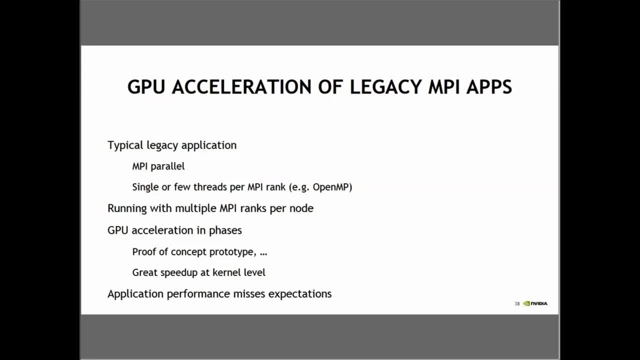 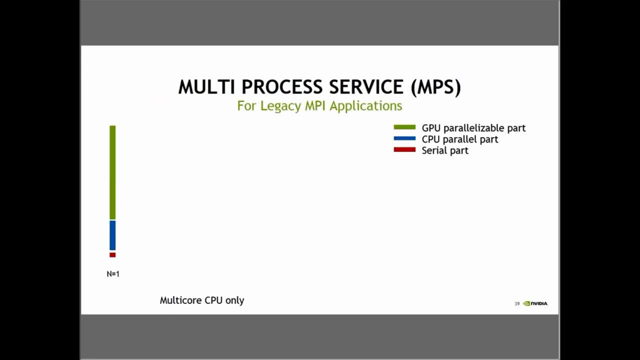 is in the proof of concept or just got started and you get a great speed up at kernel level but your application performance misses expectation. So your performance might look like that You have with one rank. you have kind of this profile: You have a red serial part, a blue CPU parallel part and a green GPU parallel part. 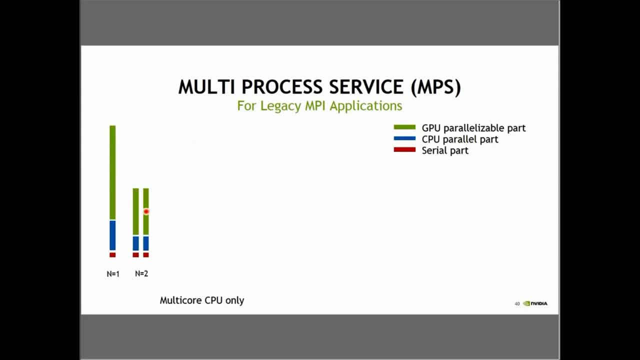 If you scale that on multi-core CPU, the CPU parallel part and the GPU parallel part both scale with the number of CPU cores you use, so that you're getting a nice speed up, And if you go to the GPU you can only use one MPI rank. 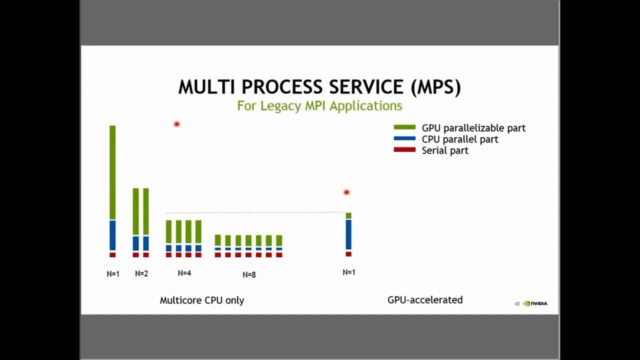 Okay And you'll see a significant speed up of the GPU parallel part, but you're slower than the CPU version because you're not scaling for the not GPU parallelized CPU parallel part And the multiprocessor is MPS, or also known as Hyper-Q for MPI. 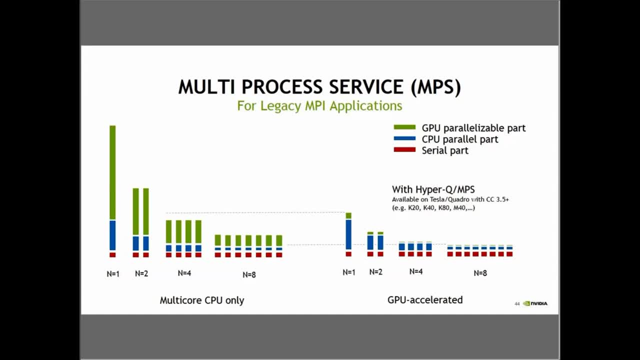 And then we'll see you to just do that and just launch multiple MPI ranks per GPU, So that the MPI ranks share a GPU and you can also benefit from the multi-GPU scaling and therefore also getting a full application speed up on a full node. 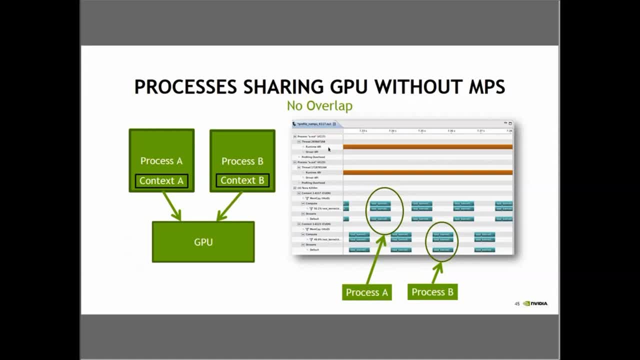 So there are some other benefits of MPS that I want to highlight. First one is: you can share a GPU also without MPS, which is not recommend, but you can do it. Then every process will have its own context, Okay, And a GPU can only serve a single context as a time. 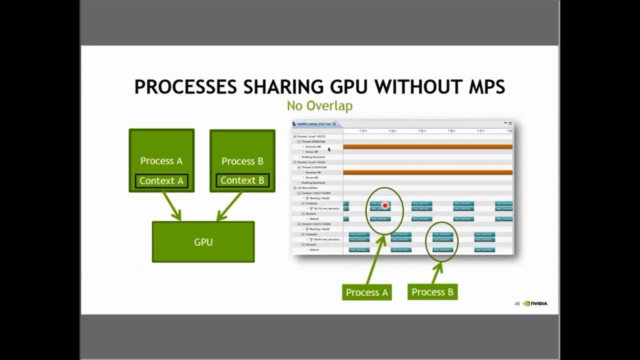 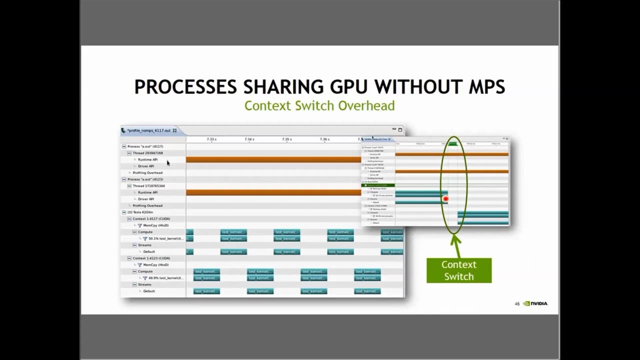 So they would execute the kernels one after the other. So first the context from process A would execute the kernels and then the kernels from process B would be executed, And between the two we have a context switch. So even if the kernels are so small that they're not, 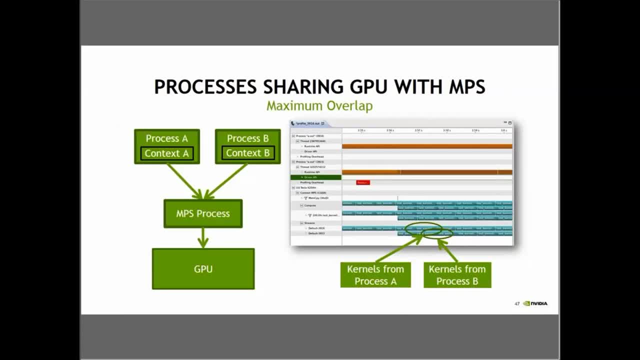 Occupying the full GPU. this would happen With MPS. the two processes are sharing a context on the GPU. We are the MPS daemon and therefore the kernels of both processes can run concurrently if insufficient resources are available, speeding up the application. Furthermore, we don't have any context switch overhead. 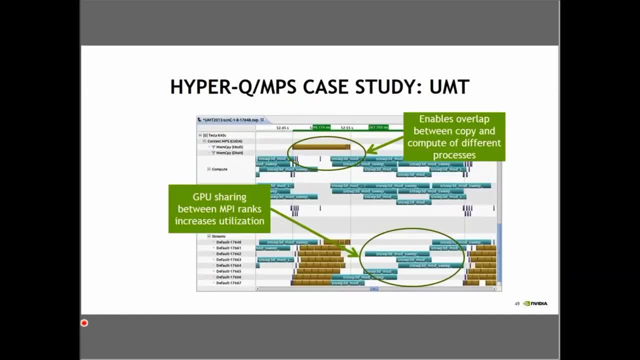 Okay, And to take a look at a case study, UMT. we, as already said, your small kernels of different MPI rings can run concurrently and increase GPU utilization, And also you get overlap of copies of one MPI ring with compute of different MPI rings. 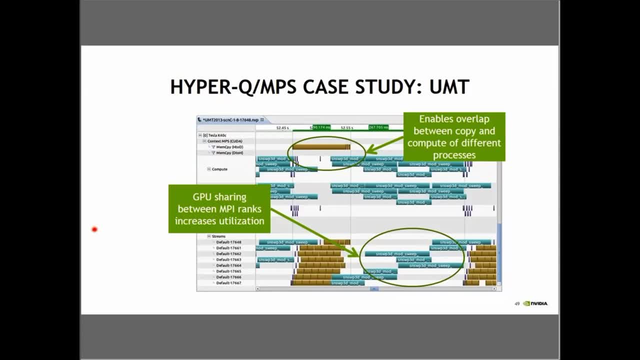 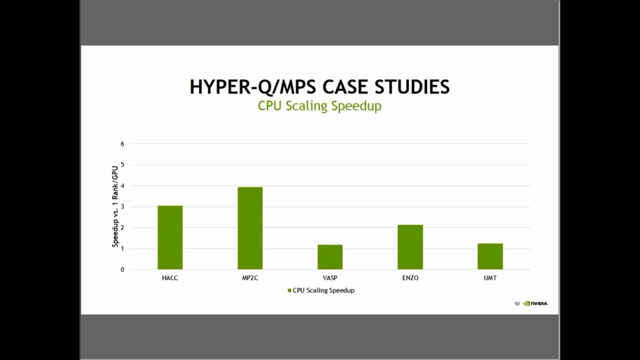 So let's take a look at a few case studies and the effect on that. So what I did here is measured the speedup one get by sharing a GPU without MPS, So essentially how much faster the application runs with using all CPU cores and sharing. 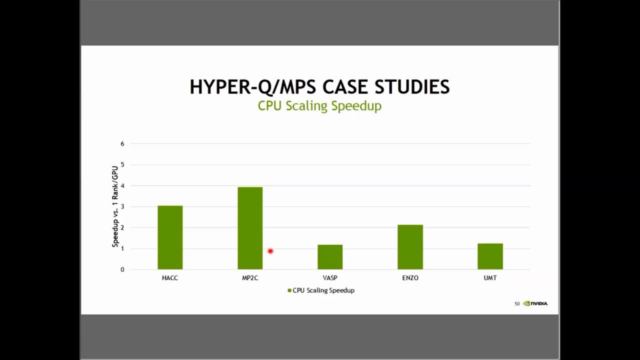 a GPU without MPS And you see that for these applications the speedup, depending on if they already support threading or not, is quite significant. If we add MPS and avoid the context switching overhead and allow overlap of work- both different MPI ranks running on the same GPU- we get an additional speedup. 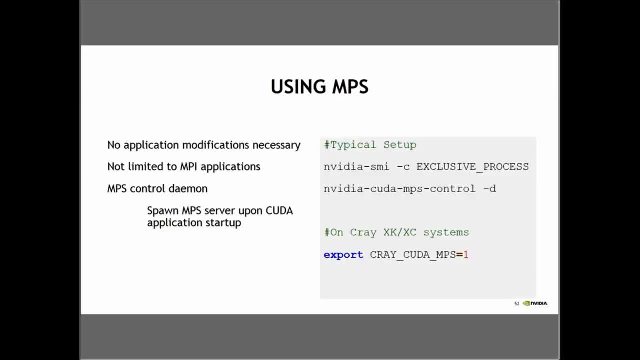 So how can you use MPS? So you don't need to do any application modifications, You just need to start your application a little bit different. It's not limited to MPI implementations, So, and what you need to do is you're Okay. 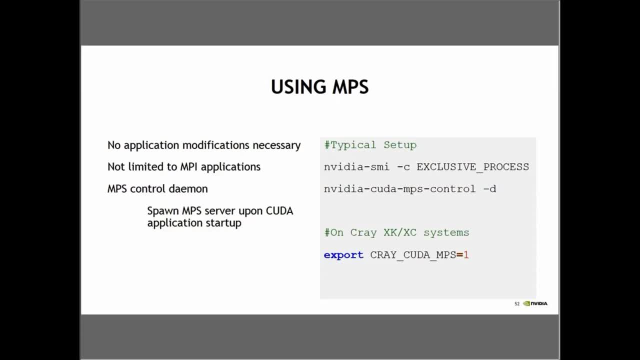 So what you need to do is you just need to start multiple MPI rings per GPU. If you control the GPU affinity with a model operation like I have just shown, that will automatically then assign multiple MPI rings to a single GPU And before that, spawn a MPS control daemon which automatically spawns an MPS server when 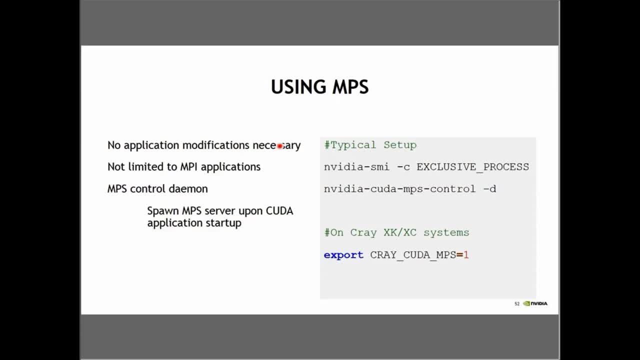 an CUDA application is started. So a typical setup would be to set the GPUs to exclusive process mode And then start the NVIDIA CUDA MPS control daemon. This is a manual setup On many clusters. they provide a different way to start up MPS. 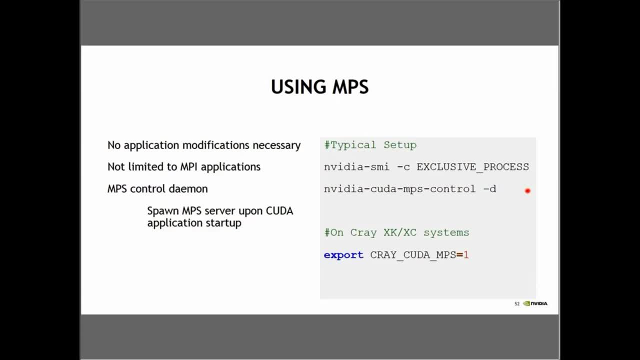 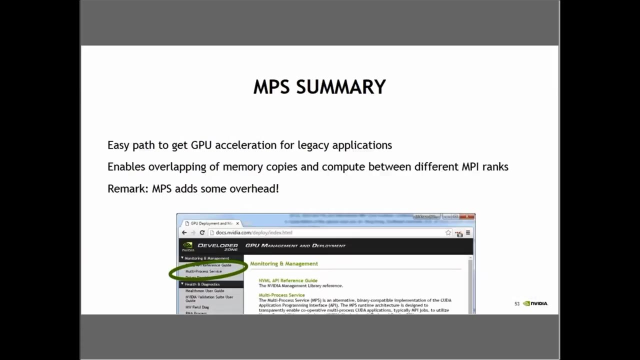 For example, we have job properties, or so One example is on Cray systems. You just have to set the environment where we have a Cray CUDA MPS to one And then MPS is automatically started for you. Okay, You can find more information about MPS on docsnvidiacom. slash deploy, slash index dot. 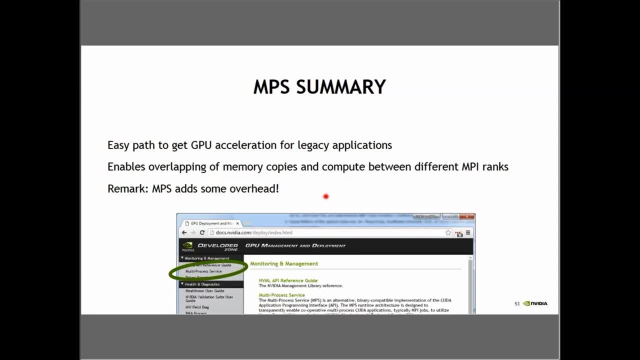 html. I want to summarize that it's an easy path to get GPU acceleration for legacy applications. It enables overlapping of memory copies and compute between different MPI rings. So you might think, oh, I want to always start that, but I would not recommend to do that. 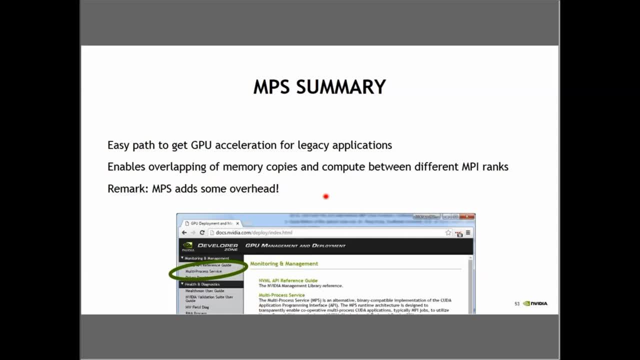 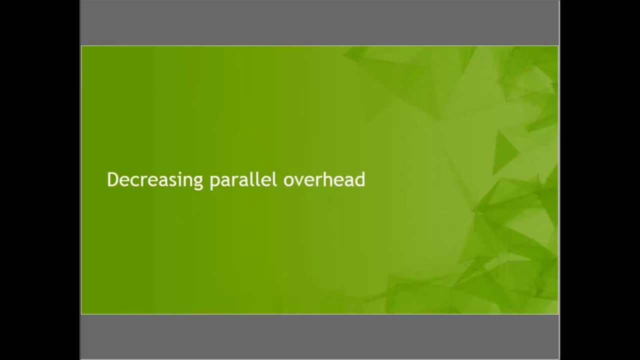 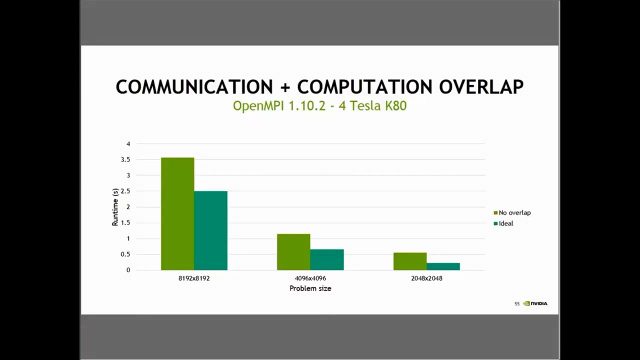 because it adds some overhead If only a single rank is using a GPU, So it should be started selectively. Okay, I see there are no questions, So I'm continuing with the last part of today's lecture: decreasing parallel overhead, Taking the Jacobi solver I have used at the beginning. 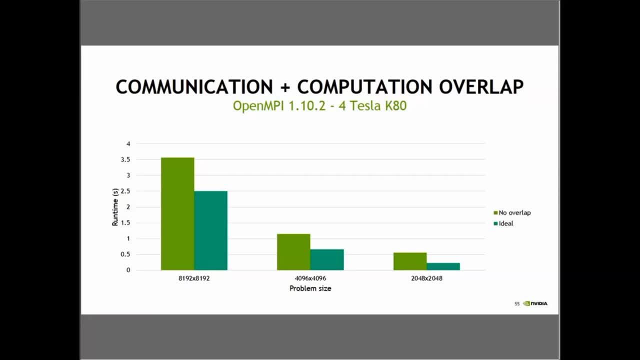 Measuring the run time for different problem sizes on four Tesla K80. We see that run time gets, of course, down with smaller problem sizes And what I compared here is, with no overlap, the run time with the ideal speed up we would expect with four Tesla K80, which, by the way, is eight GPUs. 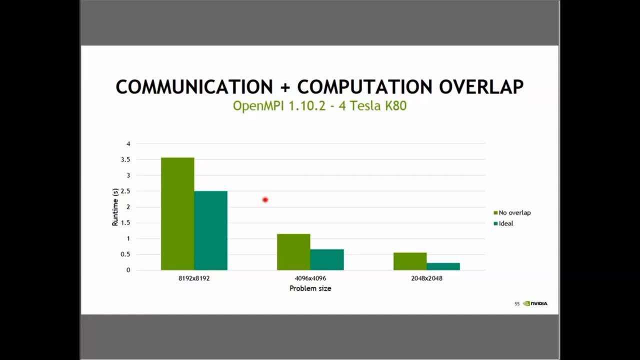 And you'll see there's quite some gap, Okay So, which is caused by parallel overhead. We don't have load imbalances here, but we need to exchange halo data between the halo data between the GPUs, which is something that is not necessary in a single GPU version. 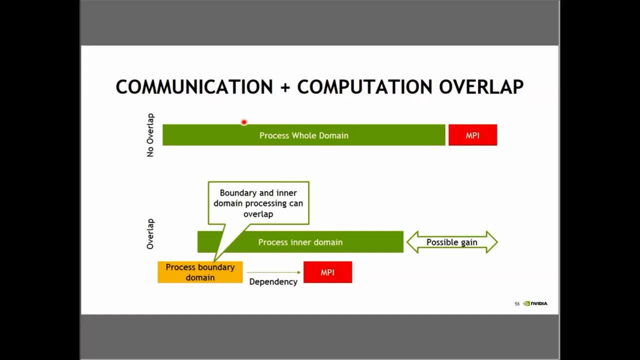 So how does it come from? So we essentially process our whole domain, then exchange data with our neighbors. So this MPI time is only done for multi GPUs And we cannot avoid the communication Because it's necessary. but we can lower the impact on the run time by overlapping. 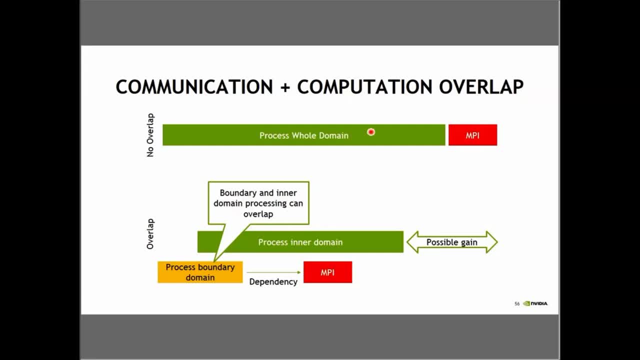 the time for the MPI communication with the processing of the whole domain, Because we only communicate the top row. we have modified at the bottom row So we could first process the parts of the domain we need to communicate with other processes And start immediately after that start MPI communication. 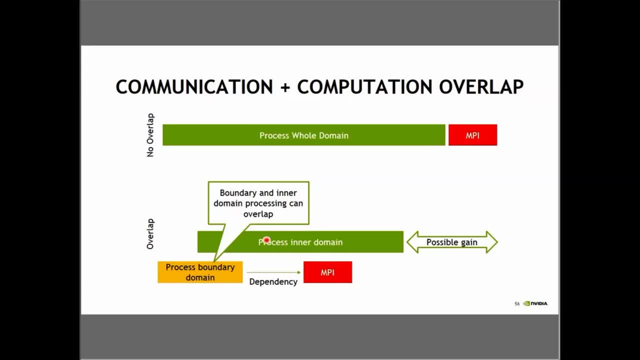 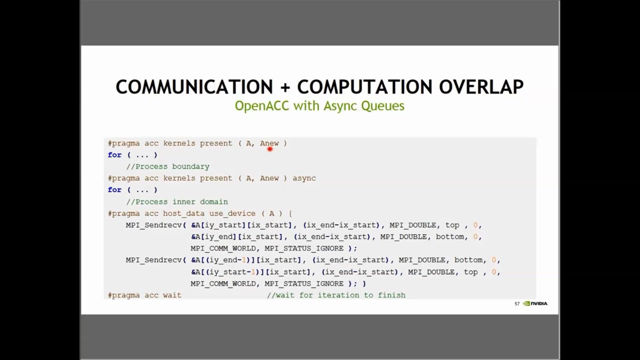 And in parallel to that then process the rest of the domain, which allows to overlap the MPI communication with processing on the GPU and therefore hides the communication time necessary. So how can this be expressed with OpenACC? So first we process the boundaries with an ACC kernel. 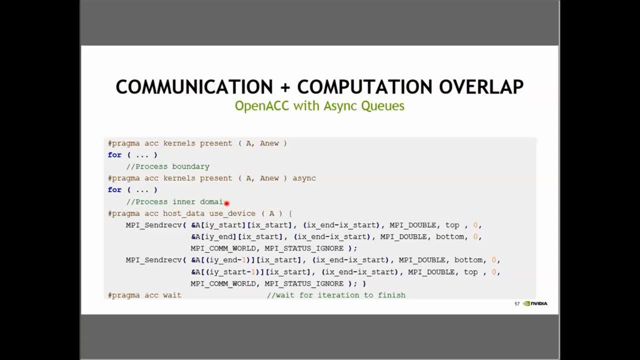 Then we start As synchronously the processing of the inner domain, So the control immediately returns to the CPU after launching this kernel. And then we carry out synchronously the MPI communication And at the end wait for our as synchronously processing of the inner domain to finish. 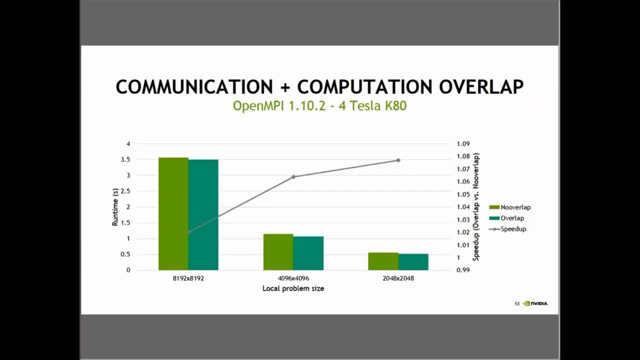 So that's the impact on the example application. You can see that for the speedup is not that large. for the very large grid because they are, the relative run time share for communication is not that large But it increases the. but it's quite some significant if you look at smaller problem. 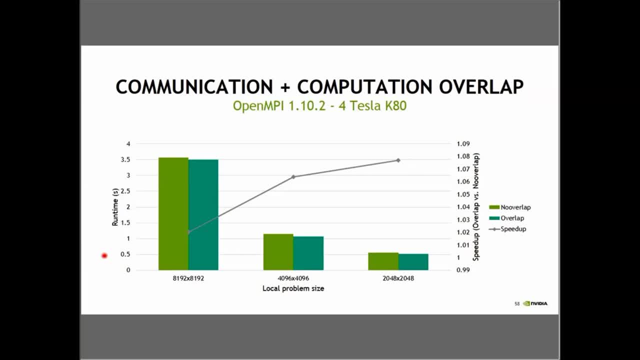 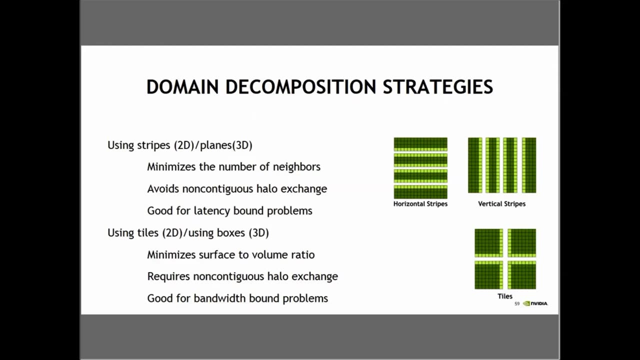 sizes where communication plays an important role. Okay, that is about hiding communication time. Another thing to increase, To decrease this parallel overhead is to lower the amount of data you need to exchange, And for the example I presented, we used horizontal stripes. 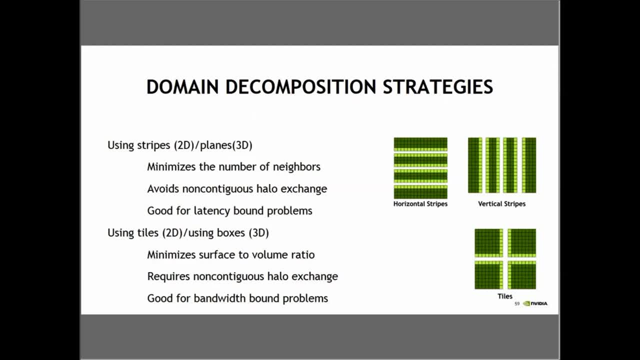 And if we run with many processes, these domains get thinner and thinner, But the boundaries, the data we need to communicate across the boundaries, stays the same. So I want to introduce different ways to do a domain decomposition. First of all, we need to do a domain decomposition. 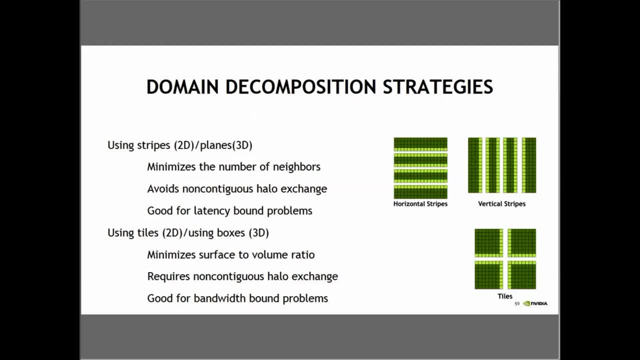 And the first one I already said, is horizontal stripes, or vertical stripes in 2D, or planes in 3D, which minimizes the number of neighbors I need to communicate to. For example, we only need to in 2D. each GPU needs to only compute with two other GPUs. 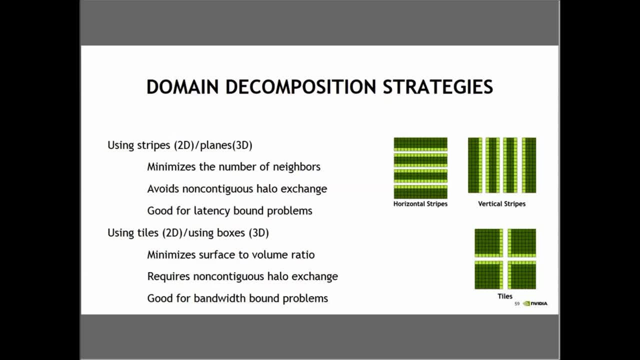 And it can avoid noncontiguous halo exchange because we have in C we have row major order. So this is the order. Okay, The halo can be sent in one time contiguous message And in Fortran we can use vertical stripes and can use the column major order to send. 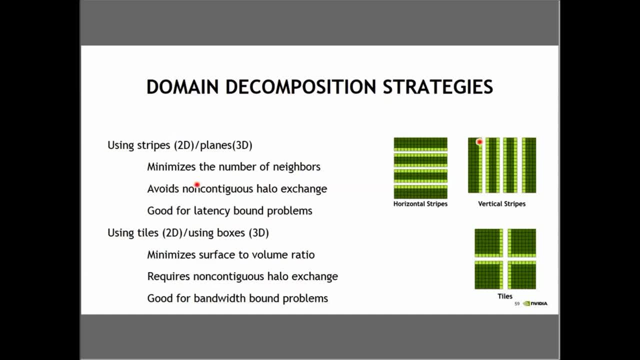 the halos also in a continuous message, which is therefore, this is best for latency bound problems. An alternative to this is using tiles or boxes in 3D and communicate, And then we need to communicate with up to four neighbors, or top, left, right and bottom. 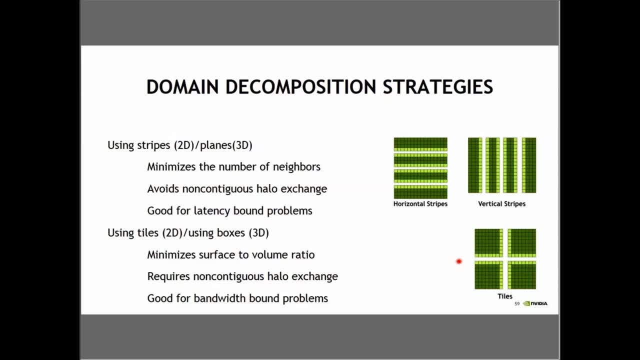 And this strategy minimizes the surface-to-volume ratio but has the downside that we need to communicate noncontiguous halos, so the columns in case of C and the rows in case of Fortran, And therefore we need to. we have a little bit higher parallel overhead, which only 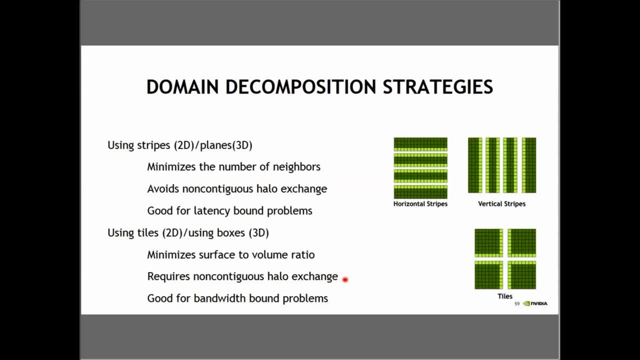 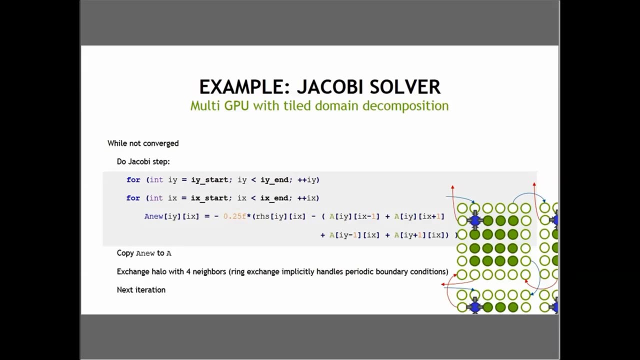 pays off if the communication is actually bandwidth bound and we really gain something from communicating less. So how is the 2D domain decomposition applied to our multi-GPU Jacobi solver? Okay, We know not only dividing our domain in stripes, but in tiles. 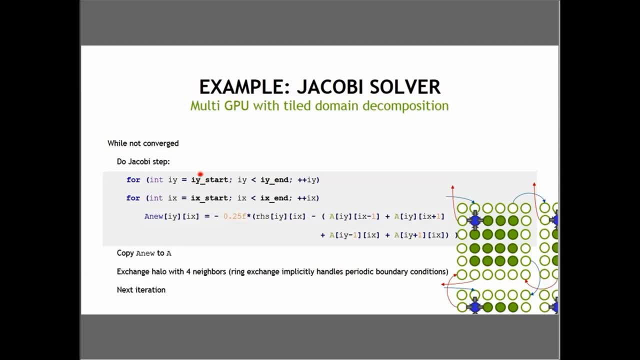 So we are computing from row AY start till row AY end, and furthermore, also only from column AX start till IX end. Then do the same One. YouTube Cobi, step on these rows, copy A to a new, and now we need to exchange the. 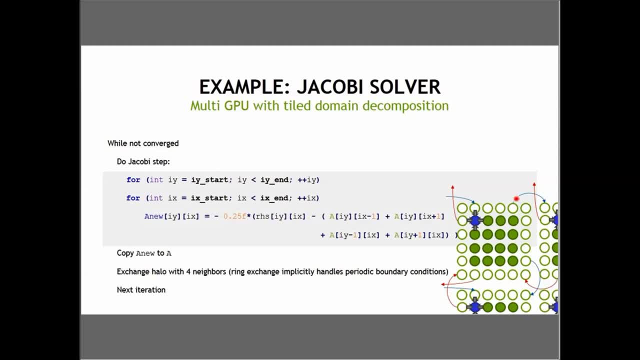 halo with 4.. These are our neighbors. We need to send our last modified column to our right neighbor, our last modified row to our bottom neighbor, and so on, And then start the next iteration. Okay, Besides computing, which is the start and the end row, and an important thing is how. 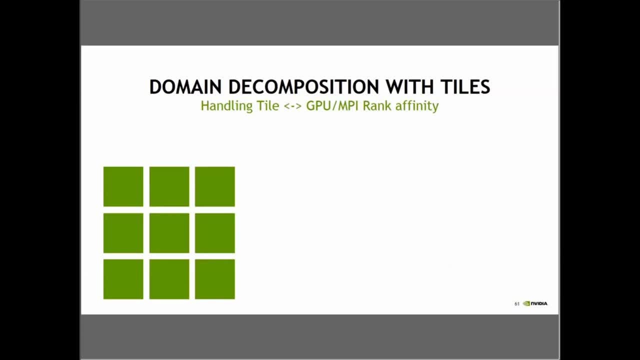 to handling tile GPU MPI rank affinity, because we now have- taking example now by a three by three- tile domain decomposition and so we would to calculate our left and right neighbors and the top and bottom neighbors. we would like to have two-dimensional ranks. 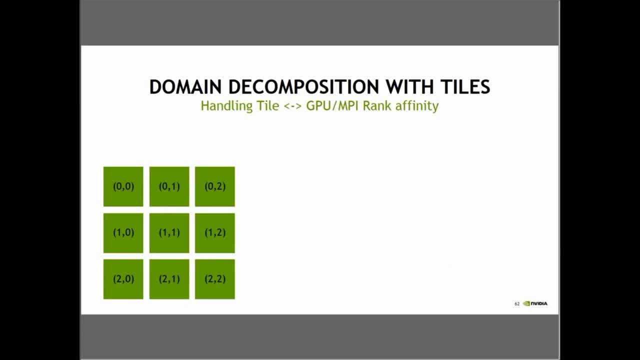 like 00,, 01,, 02, and so on. However, MPI com rank and com size only gives us 1,, 2,, 3,, 4,, 5,, 6,, 7, 8.. And so how do we map these two? 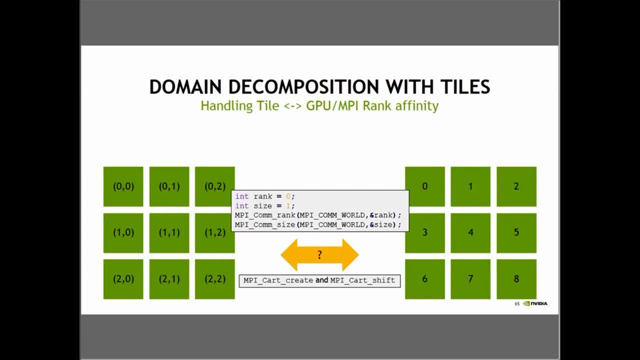 The MPI standard provides Cartesian communicators for that which you can use with create with MPI cart create and use with MPI cart shift. I don't want to go into the details of that, but rather explain how you can do this manually so that you can understand what's going on. 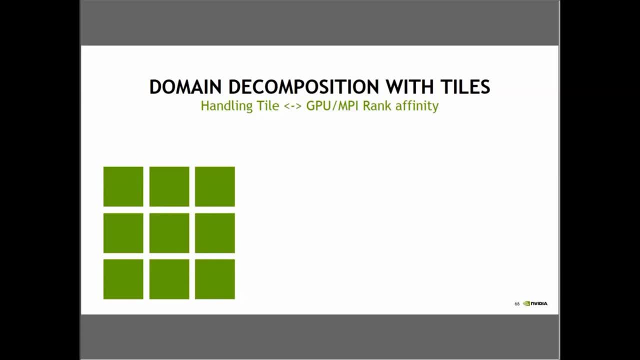 So we have our three by three tile domain decomposition. Let's start nine MPI ranks. So first thing we do is calculating our number of ranks in X and Y direction. So the size in X direction is in this case hard coded but usually would be provided. 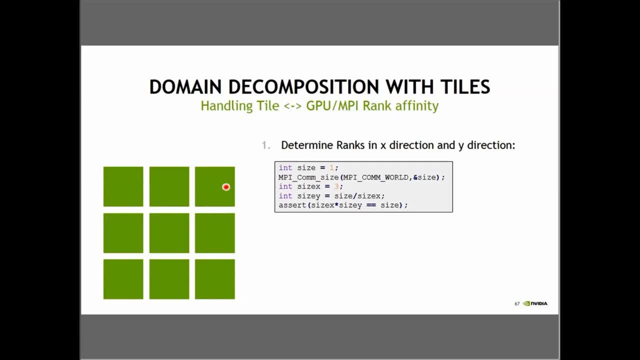 by an argument to your application. So we know how many ranks we want to have per row, per set of rows, And from that we can just, We can just divide our size, our global number of ranks, by the number of ranks per row to. 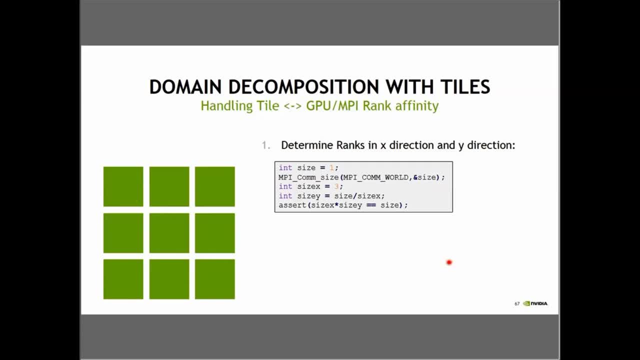 get the number of ranks per column And then just insert an to check that there are no rounding errors because we have passed wrong arguments. After that we want to map our 1D MPI rank to 2D MPI ranks And that we can just do with a. 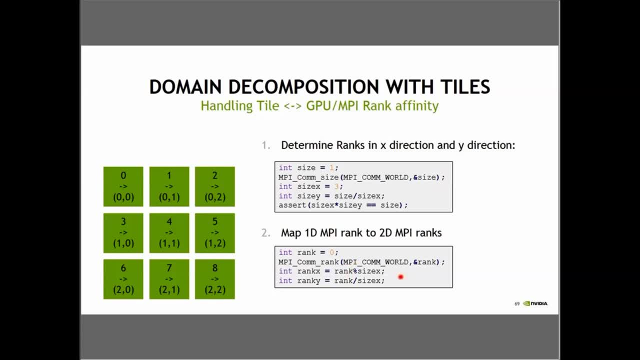 Modulo operation by doing a rank modulo size X to get the X coordinate of the tile we are responsible for, and with a divide operation of our global rank to get the Y coordinate of the tile we are responsible for. Okay, Now we have the two-dimensional. 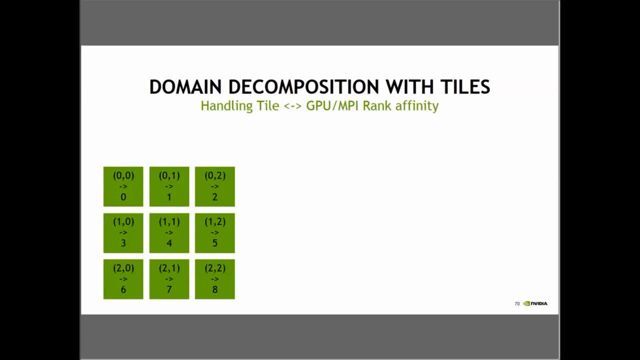 Okay, Okay, Okay, Okay. And then we have our complex Rank so that we can compute which rows and columns we are responsible for and which are our left and right neighbours. Now we need to map that back to global MPI ranks so that we can use it in MPI. 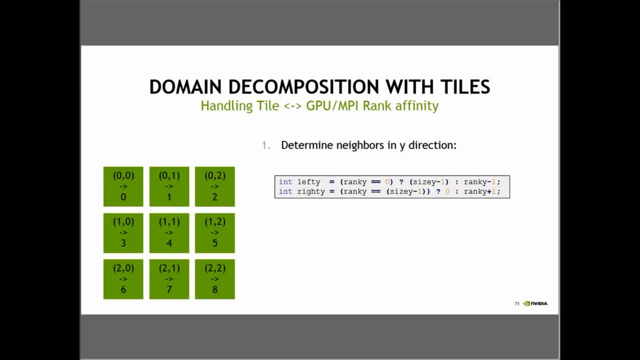 communication And for that we first To give an example: the neighbour's in Y direction. if we want to get our left neighbour, we are supposed to make sure that it comes out to the left next. So they then give us map to MPI. we need to find out that MPI rank then b. 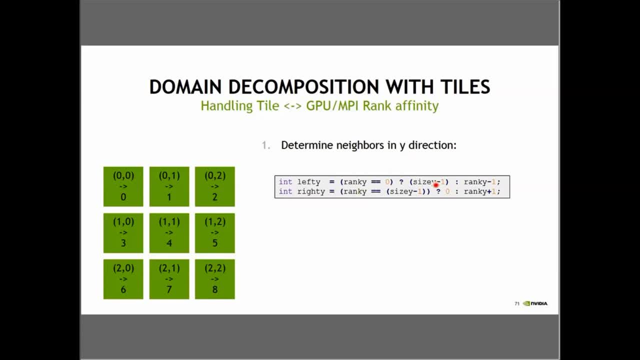 we can totally map to our жеer canalу and pick out an option that here and there is, get our left neighbor. we take our, our rank minus one. unless we are the first rank in that row, then we take the last rank on that row and the right neighbor. 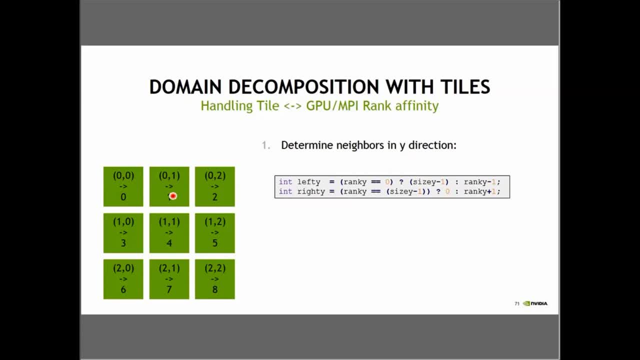 is the same. we take our rank in y direction plus one. unless we are the last one, then we take rank zero in that row as our right neighbor. Mapping that back to 1d MPI ranks can be done with the following expression: by just calculating our index in y direction, multiply it by the width and adding our 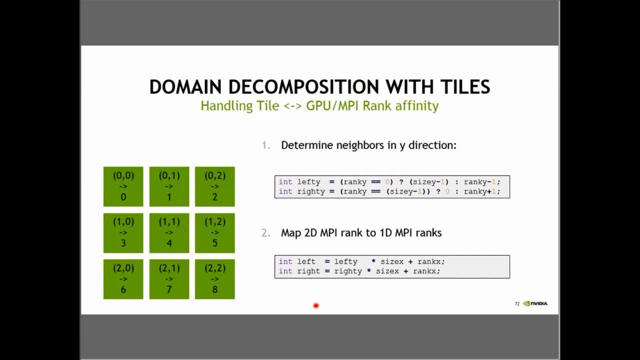 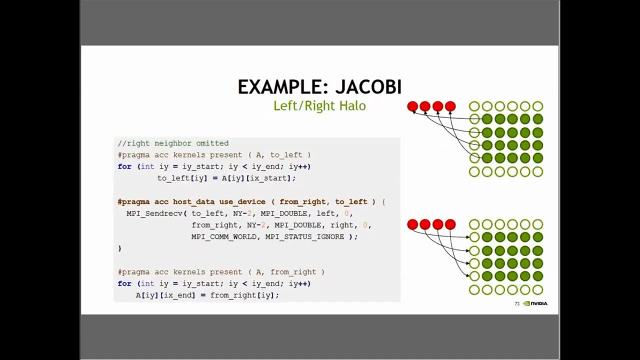 X rank and the same, of course, for the right neighbor, and then we can use these to communicate with our left and right neighbors. Since data is now non contiguous and sending various, many very small messages with MPI is inefficient, we first want to gather our non-contiguous data into a contiguous data into a contiguous. 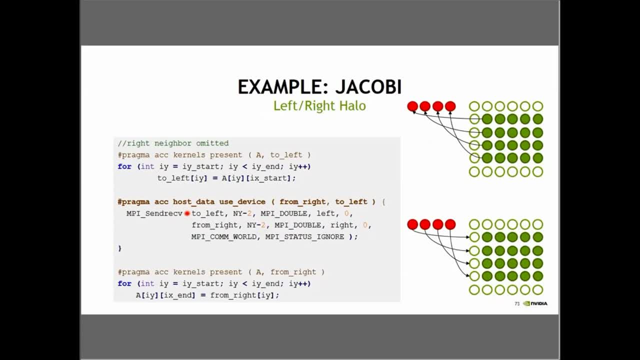 buffer which we then can send to the neighbors which are requiring them and receive to contiguous data a buffer so that we can scatter that to our non-contiguous data. Again, here, doing to come doing that manually. there's an alternative by using MPI data types, and using them might be more efficient because the MPI 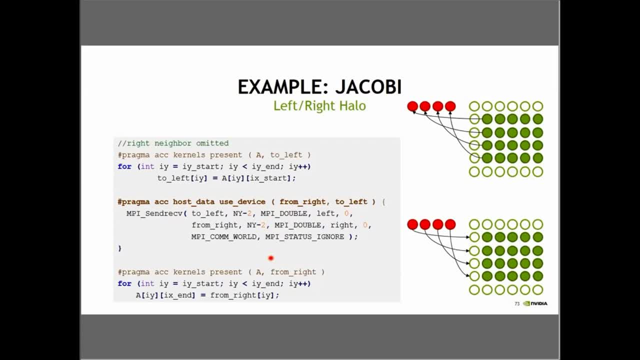 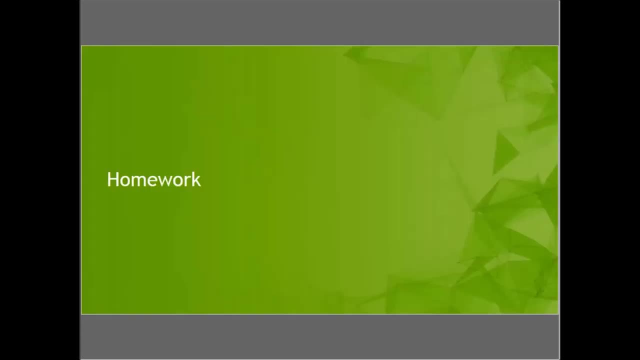 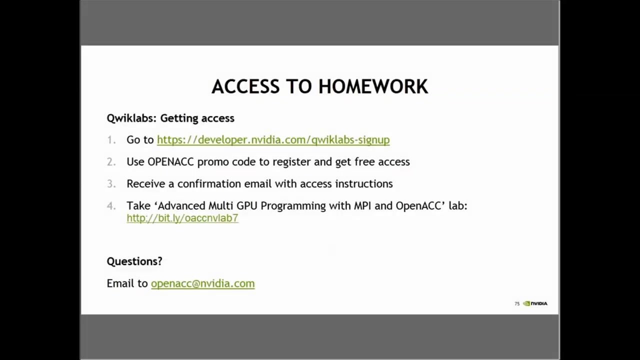 implementation could do. the can also do this gathering and scattering from you, even in GPU memory, and can embed that in its internal pipelines running more efficient. Okay, With that I want to close and happy to take more questions. I want to make you aware of the homework which you can access over Qwiklabs. Go to developernvidiacom. 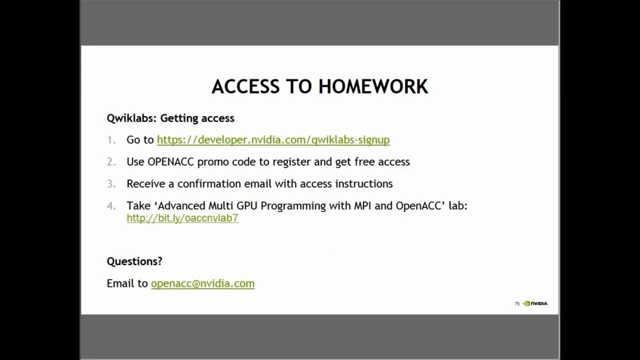 Qwiklabs sign up. Use the open ACC promo code to register and get a free access. After you receive the confirmation email you get access instructions and with that take the advanced multi-GPU approvals. You can also use the open ACC lab by using the open ACC lab. 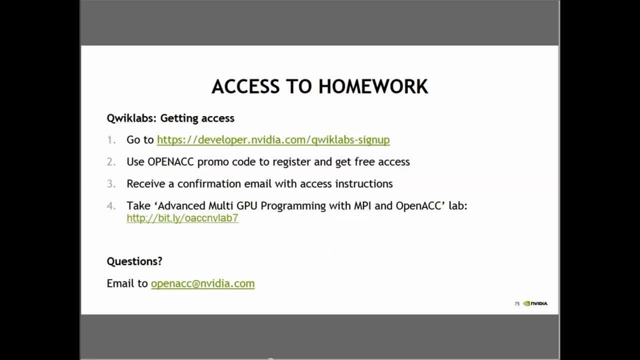 Okay, let me look at questions. There was one question: Is open ACC supported on Azure AWS? So open ACC requires an open ACC compiler. so if you're So, open ACC requires an open ACC compiler. so if you're have one, if you install one on your Azure AWS instance. 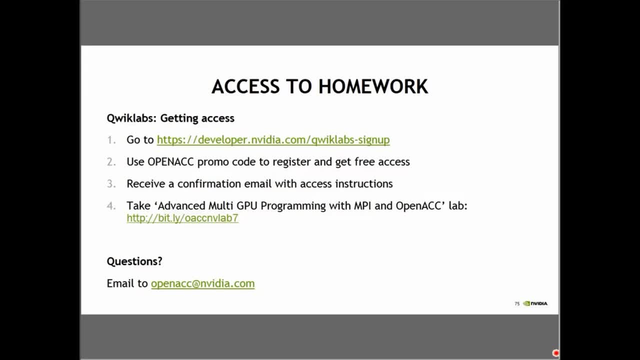 you can use OpenACC there. Actually, the Qwiklab is running on an AWS cloud instance and we have the OpenACC compiler running there, so you can even try that in the homework. On slide 44, there's a question. 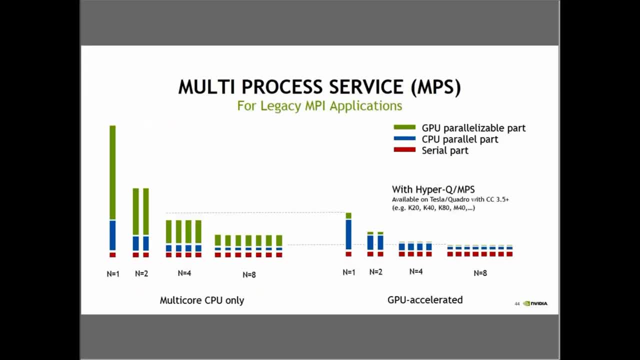 On slide 44, N on the chart. N represents a number of processes or multiple core GPUs. N represents a number of on this slide, N represents a number of MPI ranks and corresponds to the number of CPU cores used. So N1 means one single-threaded MPI rank running. 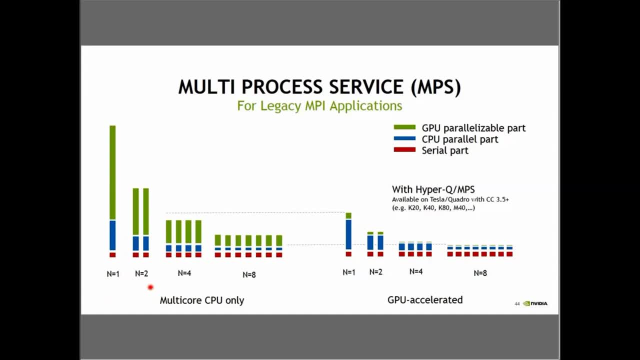 on one CPU core. N2 means two single-threaded MPI ranks running on two CPU cores. And there's one more question: Do all these examples assume that all the data can fit on the GPU simultaneously? Yes, The problem is assumed to fit in the aggregate GPU memory. 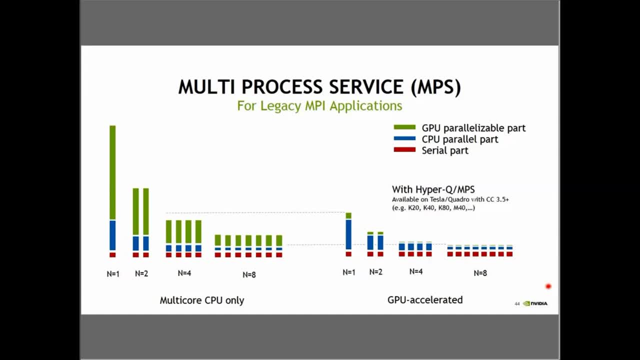 of all participating GPUs. Then there's a question with if the PGI Fortran compiler can be used with MPI-RAN and MPI-CC. Yes, the PGI Fortran compiler can be used with MPI. You would also use MPI-RAN to start your application. 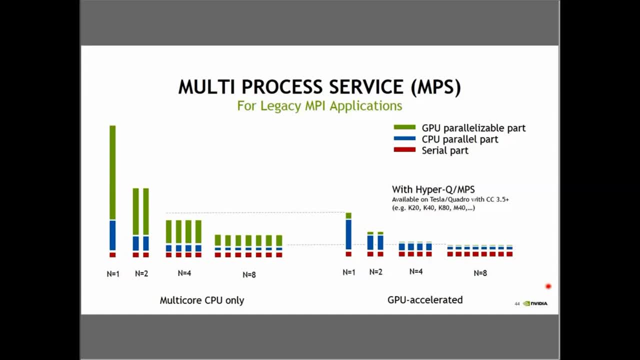 but you would use the MPI-F90 compiler wrapper instead of the MPI-CC compiler wrapper to use the to assess the Fortran compiler. There's one more question: Is this straightforward to screen data to the GPU with OpenACC? Probably a follow-up to the question, if 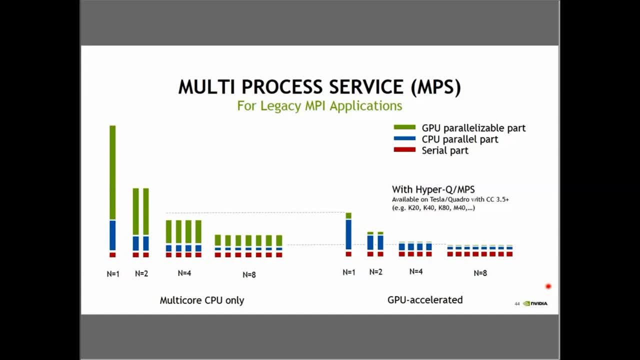 if the data needs to fit into the memory of the GPU. Yes, you can do that with as-in clauses and as-in for as-in chronos data transfers. This one was. this topic was covered in the class number four of the last OpenACC course. 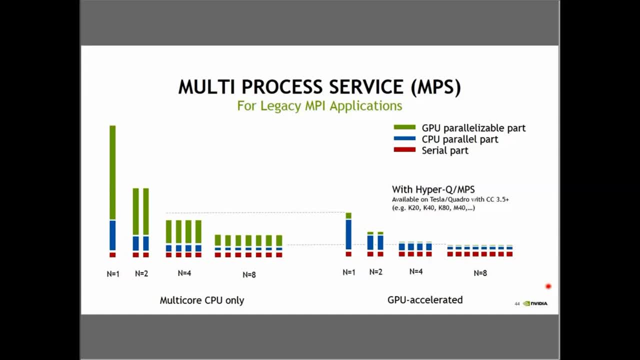 So if you're interested in that, you could either watch a recording of that or take the lab covering that topic. Another follow-up question on that is: does if screening works with MPS? Yes, streaming also works with MPS. You just have to consider that if you share a GPU. 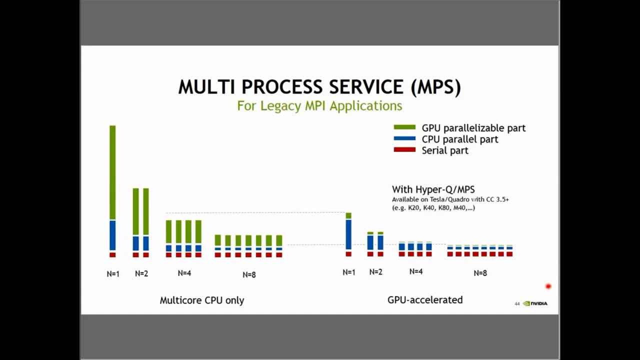 with multiple MPI-RANs there are just more processes competing for GPU resources. So if one GPU resources is occupying the copy engine to move data from the CPU to the GPU, it's more efficient, It's blocked for the others. Then there's a question. 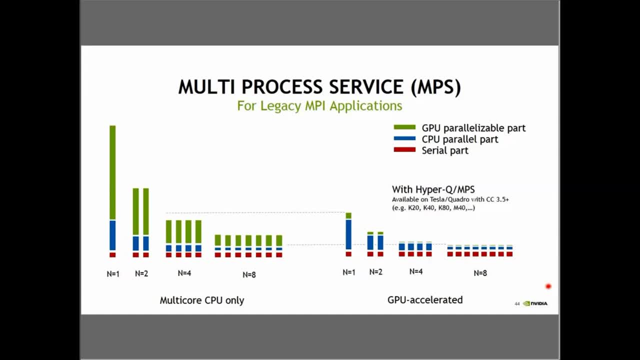 Why MPS is for legacy MPI implementation, So the it can be it's meant for. I highlighted that it is for legacy MPI implement applications because with the legacy MPI application, you probably have started to accelerate a few of the few most important routines. 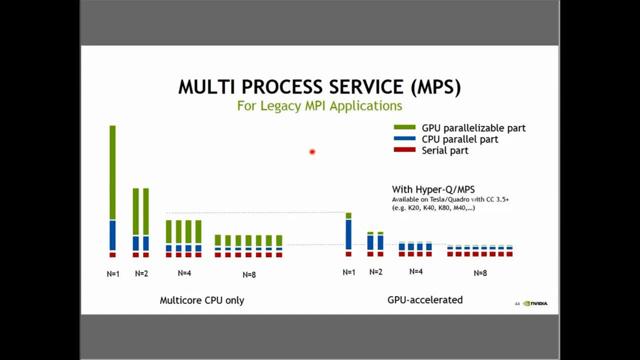 but not all of them. So you have the effect shown on the slide, on slide 44, that you're that you're getting speed up for for these routines but not for the other routines. So, and then MPS enables you to get an application speed up. 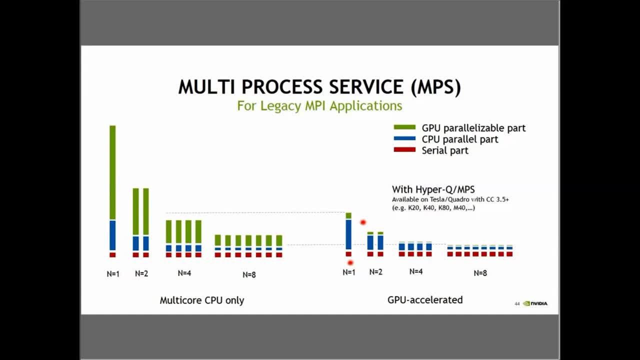 In general. if you continue, usually you would also parallelize the CPU parallel part on the GPU and therefore all of that would run on the GPU and then you would no longer use MPS and just start one MPI rank per GPU. There's a question. 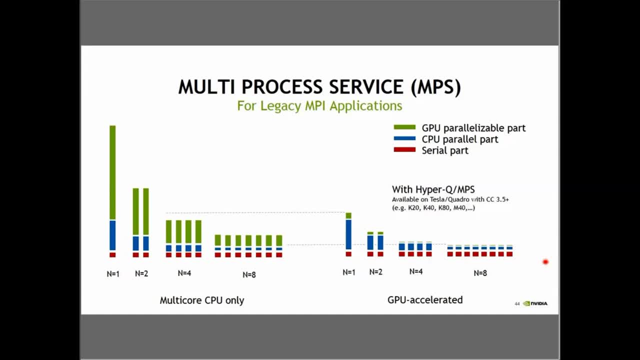 There's a question if its operations run on a GTX 960 and a GTX 730 on Linux, on a Core i7 on Linux, yes. however, you would likely get load balancing issues and, compared to a Tesla, the CUDA WAMPI will not use GPREC peer-to-peer transparently for you. 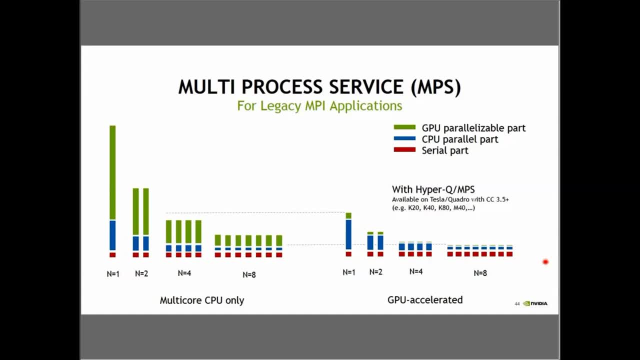 Then there was a question: which PGI compiler version did I use and if there's a difference between recent versions For the code presented here. I'm not aware of any major differences between the recent versions and I used version 16.3 for that. 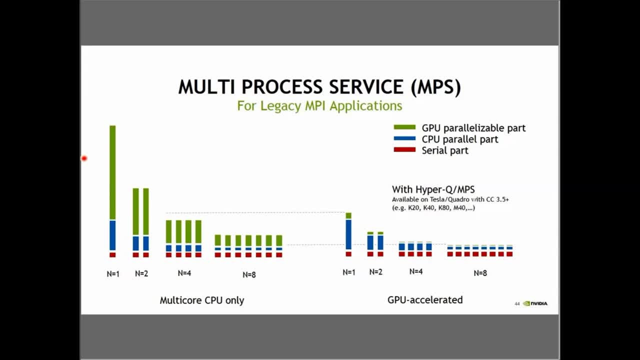 Okay, since there was a question on using that on GeForce, I want to jump to an implementation detail of CUDA WAMPI, explaining what benefit you will get from using a CUDA WAMPI, in addition to the ease of use by just passing in device representations. 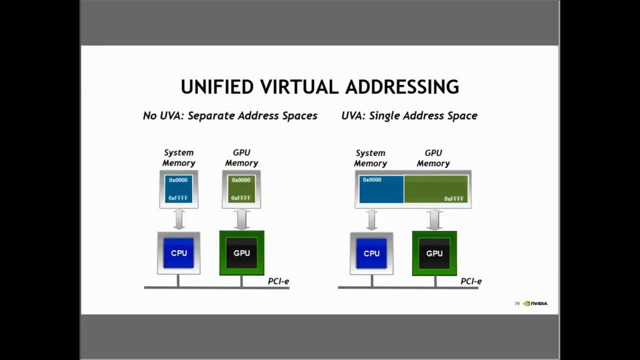 Okay. so first thing I want to shortly highlight why it works. CUDA, WAMPI and the enabling technology for that is unified virtual addressing. because unified virtual addressing puts all the memory of the CPU and the GPU in one large single address space. 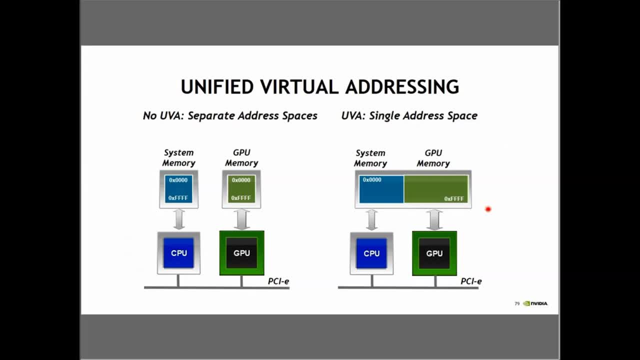 So that you can identify where a pointer points to from its values. If you would have no unified virtual addressing, you would have two address spaces for the CPU and the GPU- and you could have one pointer value which is valid on the GPU and on the 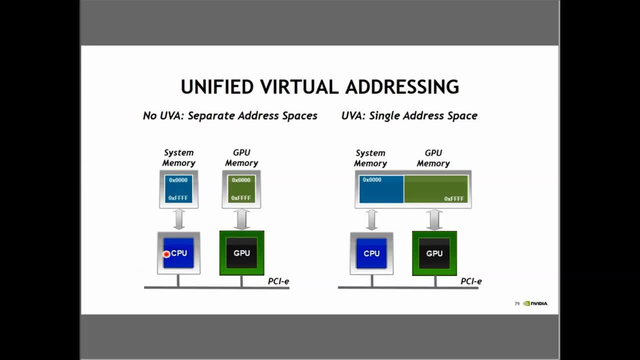 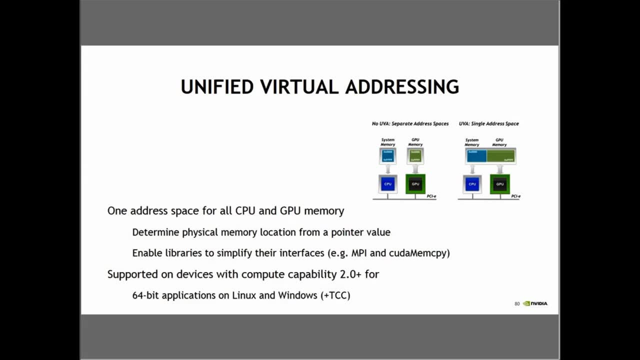 CPU but points to different memories. With unified virtual addressing, for example, a library can query the pointer if it points to GPU. If it points to GPU memory or to CPU memory and depending on the physical memory location, it can take different execution paths. so in case of MPI, if it gets a GPU memory, it 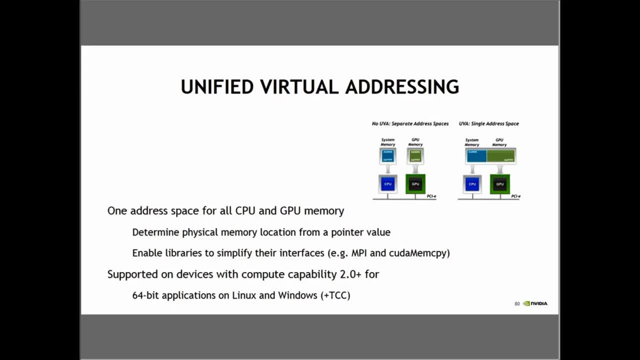 can start a host staging pipeline or use a GPU direct path, which I will introduce in a second, to transfer the data and use some other methods to move the data from RAMRANG to the other, Or, if it is a host pointer. Requirement for that is a device with compute capability 2.0 and a 64-bit application, which 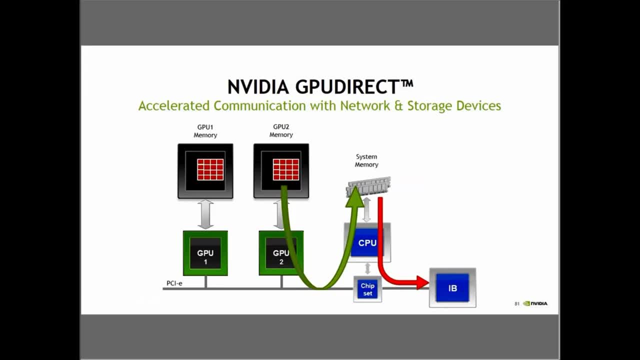 should be pretty much everything today. Okay, that's the enabling technology for CUDA-Aware MPI, But another benefit, so how you can use it, and I want to highlight some acceleration technologies which you might have heard about: GPU direct, which CUDA-Aware MPI will. 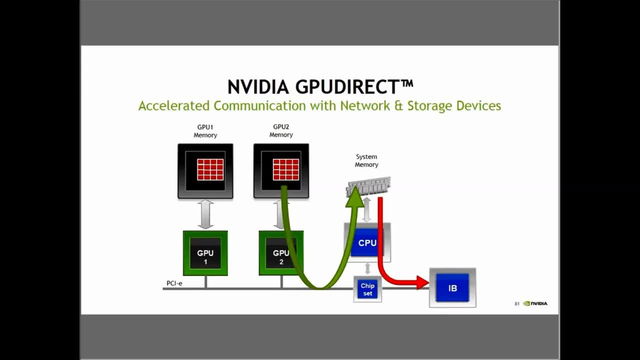 transparently use for you to speed up your inter-GPU communication. First one is GPU direct for accelerated communication with network and storage devices. That allows that an InfiniBand adapter shares a pin system memory buffer with the GPU so that the DMA transfer from the GPU can directly go to a buffer, which can also be used for. 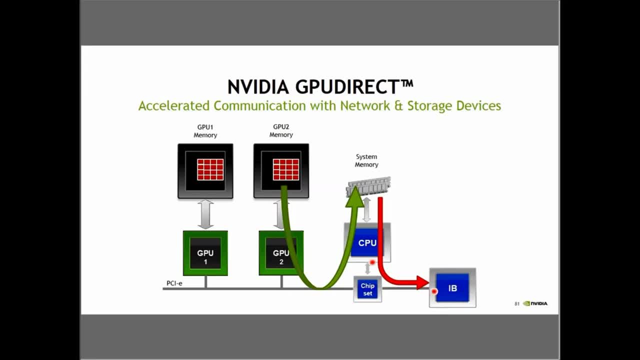 RDMA transfers to a remote node. Without this technology, you would need to have one DMA-able buffer for the GPU and one for the InfiniBand adapter, and therefore had one intermediate copy within system memory. This one is pretty much available on all systems supporting GPU direct. 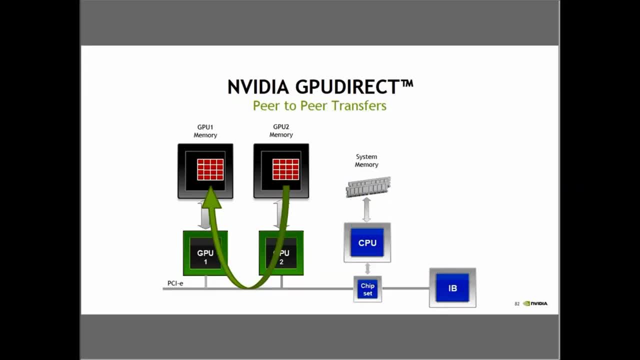 Second one is GPU direct peer-to-peer. This allows to directly transfer data from one GPU to another GPU if they are connected to the same PCI Express root complex. So without GPU direct peer-to-peer, the data would first need to be copied from one GPU. 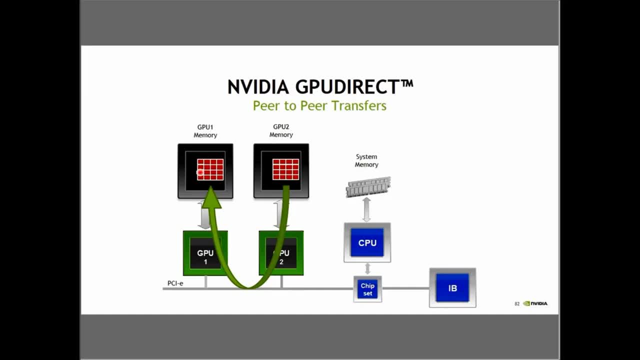 to system memory and then from there to GPU one. With GPU direct peer-to-peer, this can be avoided and it's directly sent over PCI Express bus. The third one. the last one is GPU direct support for RDMA, which allows to do the same. 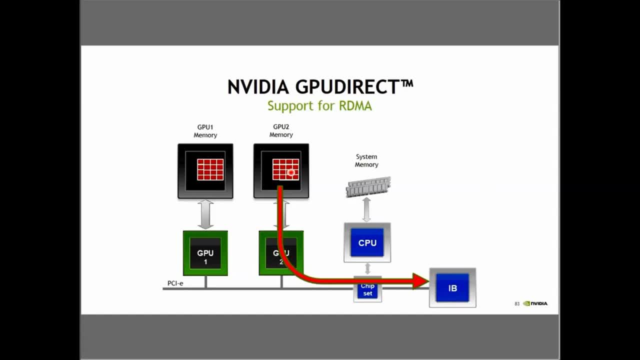 as GPU direct peer-to-peer, by sending data directly from GPU memory to an InfiniBand adapter, avoiding the staging through system memory and significantly reducing latency. What does it mean for? How does it Does it? How does CUDA or MPI use that? 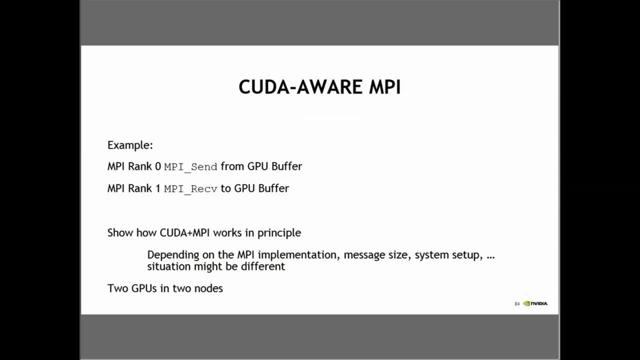 For that I want to show you a short example which says that MPI rank zero does an MPI sent from a GPU buffer and MPI rank one does an MPI received to a GPU buffer. And this shows how a CUDA plus How OpenACC or CUDA plus MPI works in principle. 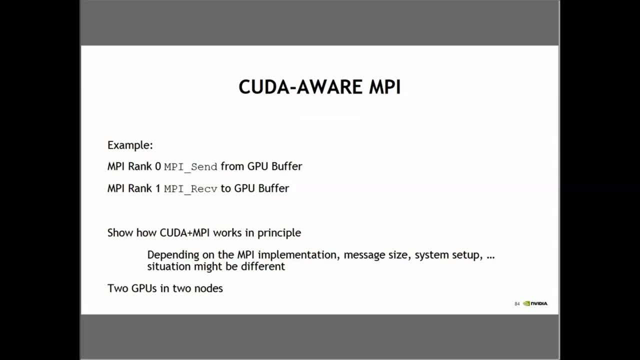 Depending on your The MPI implementation. you use the message size system setup, for example, if GPU direct RDMA or GPU direct peer-to-peer is. So this shows how, If GPU direct peer-to-peer is available, the situation might be different. 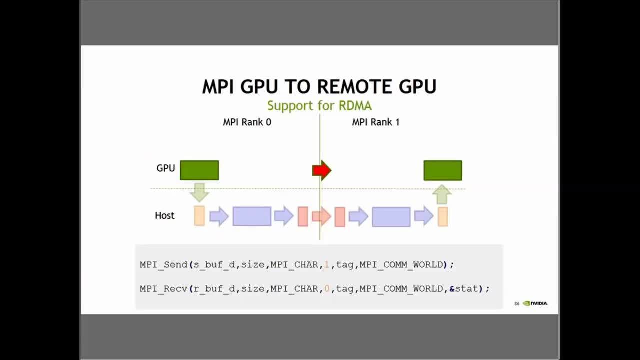 I'm looking here at two GPUs and two nodes, So let's start with the best of both worlds. if we have support for GPU RDMA, If we call an MPI send, the data is directly sent via the network and from the network to the destination GPU. 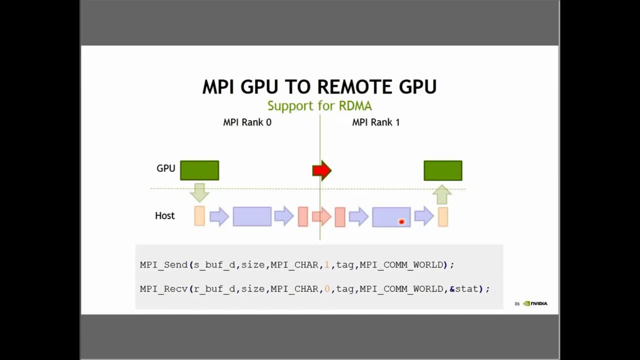 So any possibly needed host staging buffers are avoided. The MPI implementation: The MPI implementation, The MPI implementation- might decide to implement that in a small pipeline and therefore, in this case, for example, transferring it in four smaller chunks, but leading to a quite 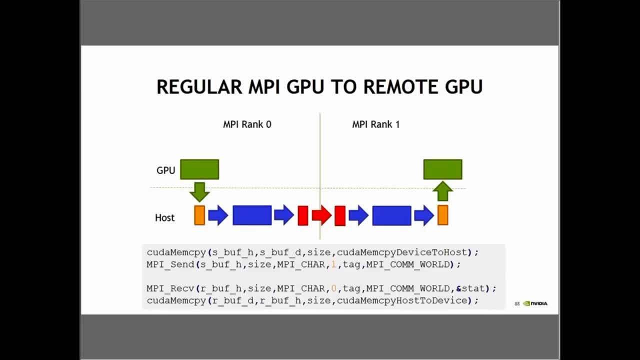 short communication time. In contrast to this, if we would use a regular MPI to send GPU memory from one GPU to the other, So we first need to copy, which would be ACC update host from the GPU to the host memory. because this copy happens with DMA transfers, so that will also involve intermediate copy. 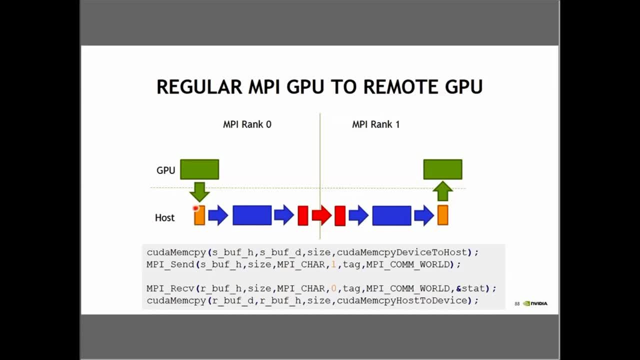 to a driver-managed staging or OpenACC runtime-managed staging buffer. until we have transferred all the data to an application-managed The application buffer on the host, Then this one can be sent. This one can be sent with MPI over the network, which might involve an ADMR-able pinned buffer. 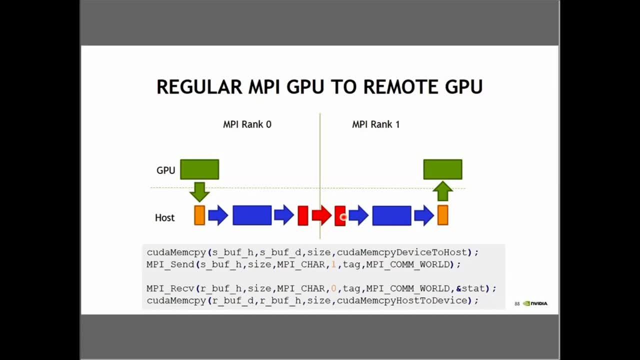 managed by the InfiniBand adapter sent over the network. We have also again the ADMR-enabled buffer, possibly the host side buffer, then the DMA buffer managed by the CUDA driver or the OpenACC runtime, and then the DMA to the GPU. 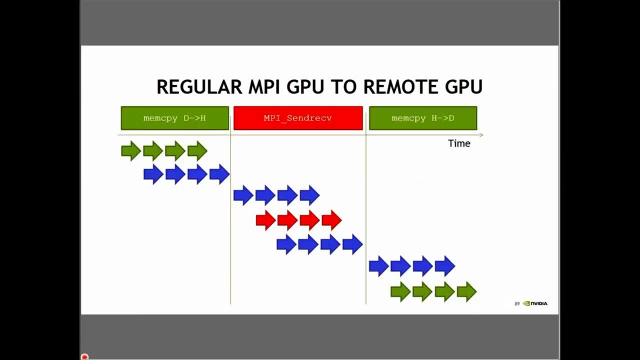 So this involves quite a few more steps. But, more importantly, After the host-to-device transfer, the pipeline is stalled before the MPI send-receive pipeline can start, and it's again stalled after the MPI send-receive pipeline, before the host-to-device. 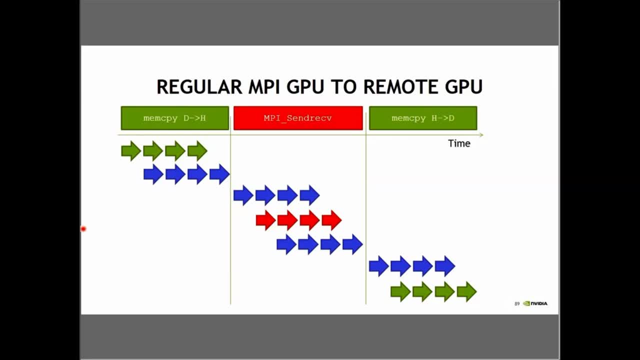 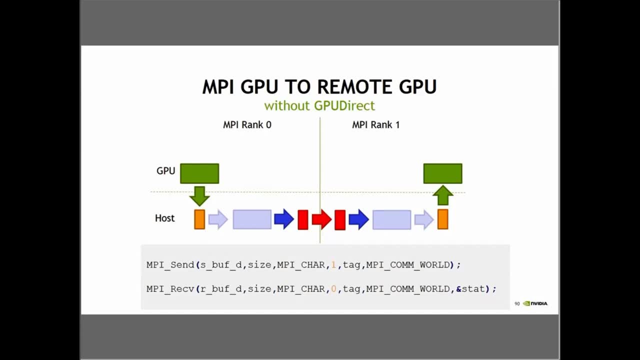 pipeline can be stalled. So one last case: If we have a CUDA WMPI but no GPU direct, We can pass the GPU pointer to the MPI directly, and then we avoid the First of all. we avoid the staging to the application-managed host buffer on the sender. 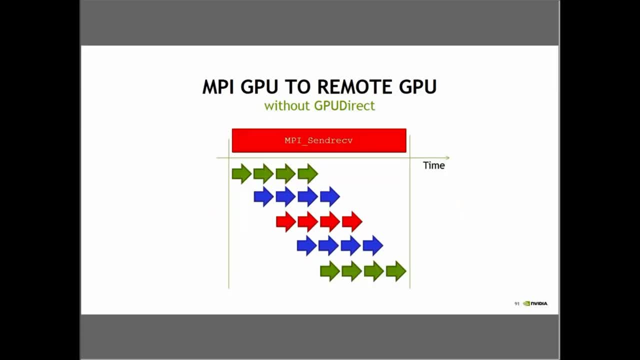 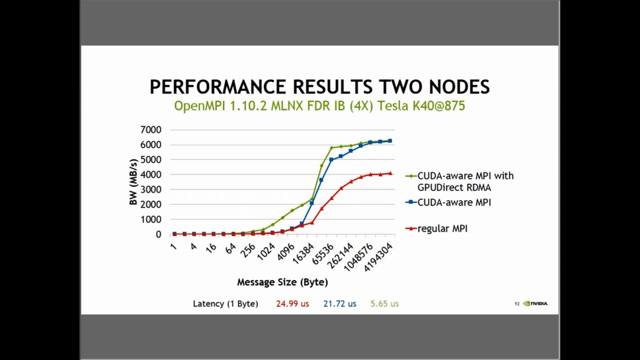 side and the receiver side. But, more importantly, everything is executed in one pipeline, so we avoid the pipeline stalls. So what does that mean for performance? Looking at the microbenchmarks- a ping-pong benchmark for different message sizes- we see that with a regular MPI and manual host staging we only reach about half the network. 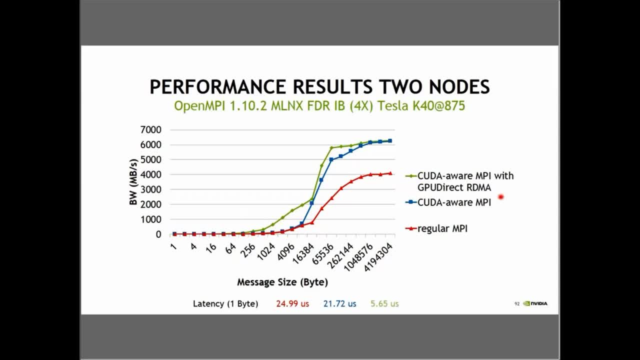 bandwidth and with a CUDA WMPI we can saturate the network bandwidth. Furthermore, if GPU direct LDMA is unable, We get a far lower latency. So that's a good example. So that's a good example of latency for GPU-to-GPU communication. 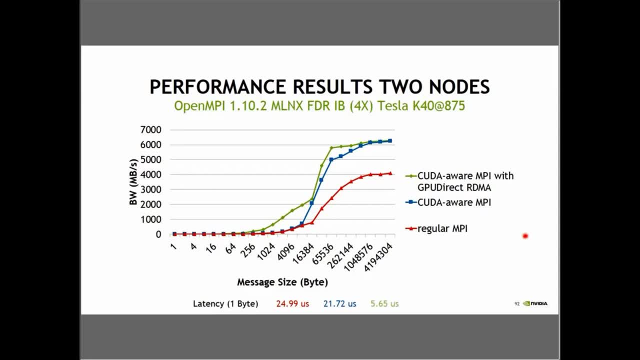 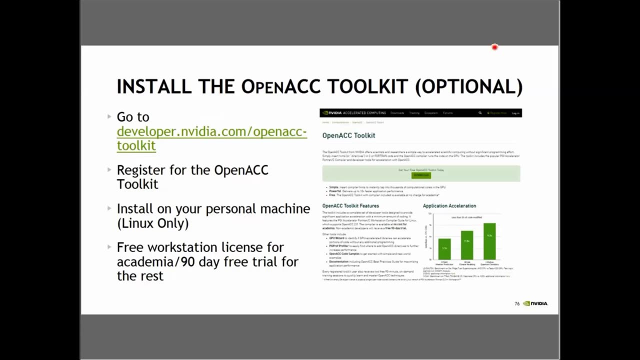 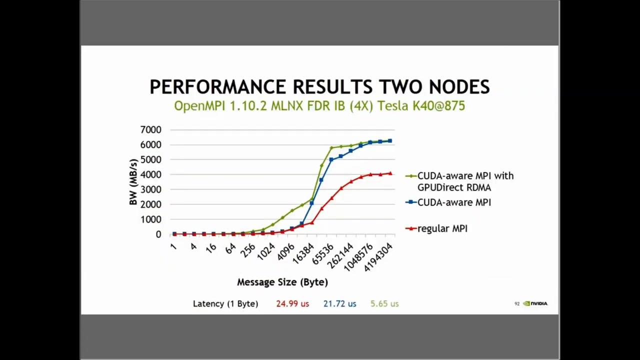 Okay, With that, I'm happy to take more questions and if there are none, I'm taking over to Julia. again, There's a question: Slide 92. If it refers to This is run on a Tesla K40, so it was connected with PCI Express 3.. 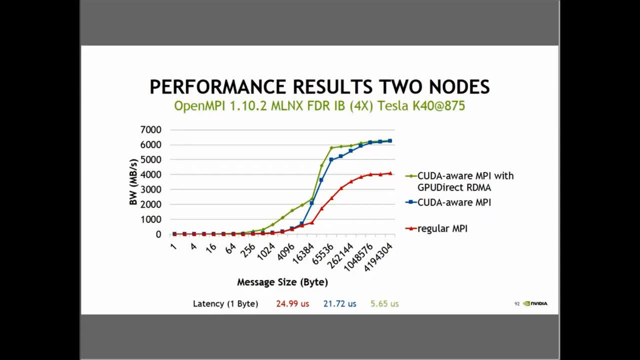 However, the Mellanox adapter is also only connected with eight lanes of PCI Express 3, and also the, Because it's sufficient to saturate the FDR-IB bandwidth. So it's using PCI Express 3 for the GPU, But we are not seeing the PCI Express 3 bandwidth because we are limited by the network bandwidth. 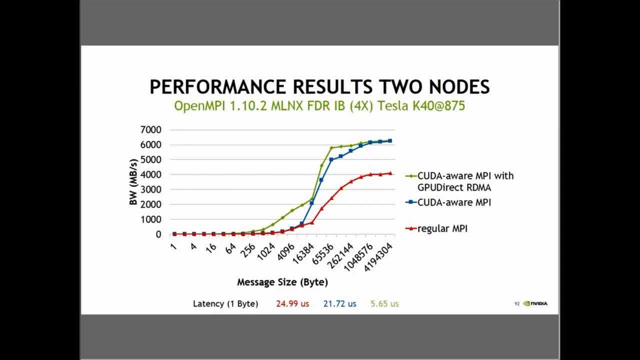 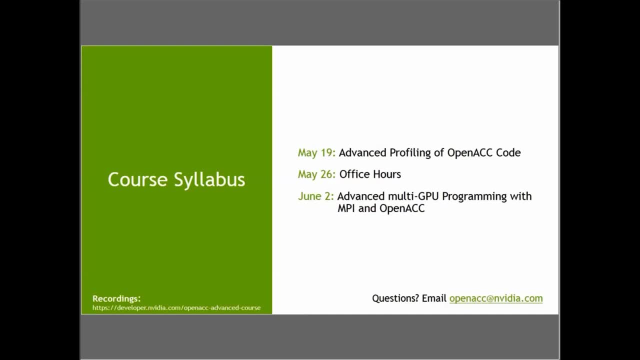 Okay, Great Thanks, Lajiri. Let's go back to the, To our questions. Sorry, Okay, So please submit the questions through your Q&A pod. We still have time. And Okay, There is one more question about CUDA WMPI. 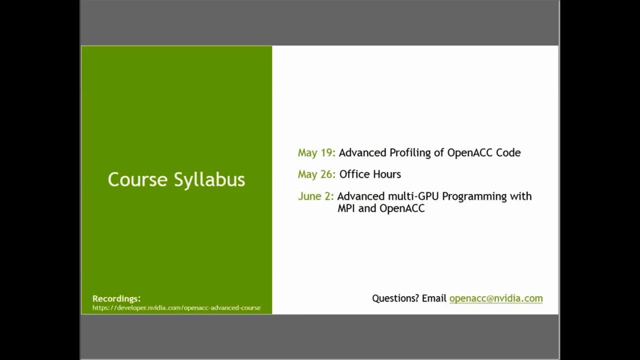 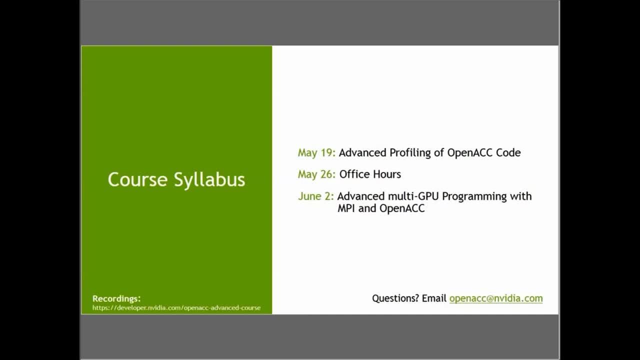 GPU-REG automatically, So it detects if In case of GPU-REG peer-to-peer. it does that always By detecting if a GPU-REG peer-to-peer part is available and, if so, uses GPU-REG peer-to-peer. 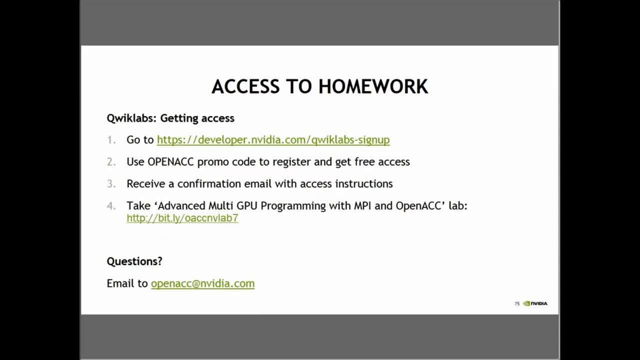 In case of GPU-REG RDMA, it's a little bit dependent on the MPI implementations. Okay MPI implementation you're using, For example, in MVA pitch. you need to enable GPREC RDMA with an environment variable. Great thanks, And let me do a couple of announcements while people are submitting. 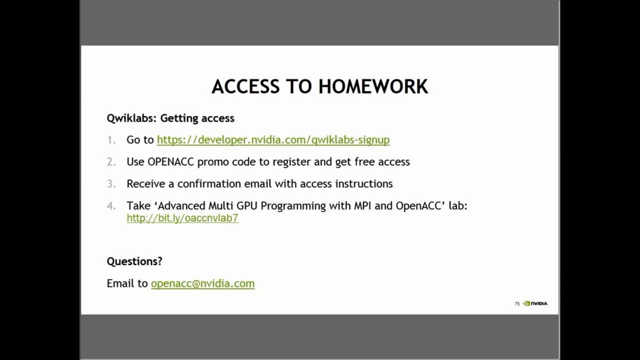 more questions. So again, one more time. just a reminder: this is the final session of our OpenACC course, of the advanced OpenACC course. We're going to be doing more courses going forward and we'll keep you updated If you have any questions. there are a lot of resources. 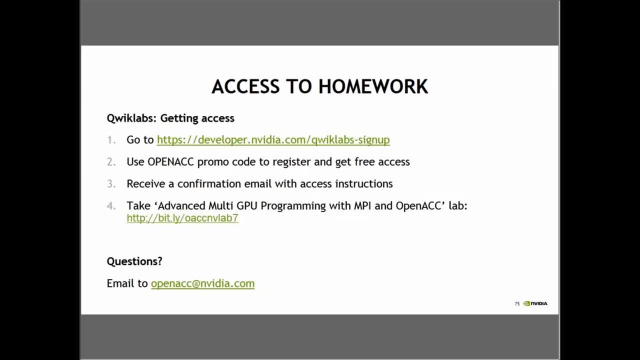 for you available. For example, you can go to OpenACC org. there are a lot of materials out there. We are also posting a lot on the Stack Overflow. You'll also have an email, OpenACC at nmediacom for your questions. If you have any ideas or any topics that you're 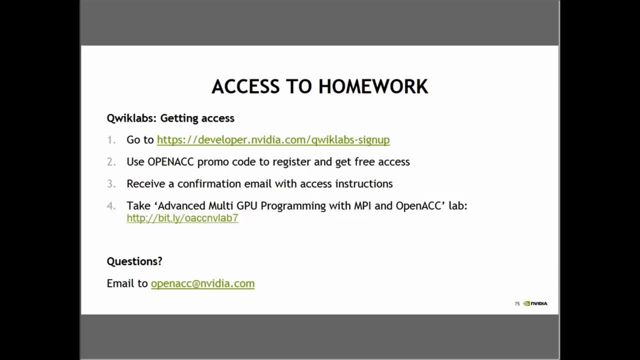 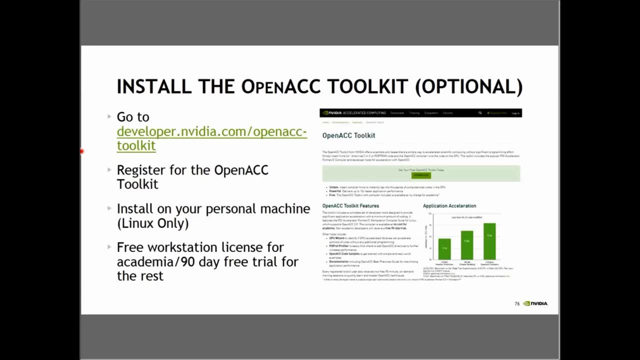 interested in to cover next time? please let us know as well. You also can download the can download the open ECC toolkit which is free of for academia. it's a free license that work on the workstation you're welcome to download it. if you're in industry, you still have an option to download it for free and use it free for. 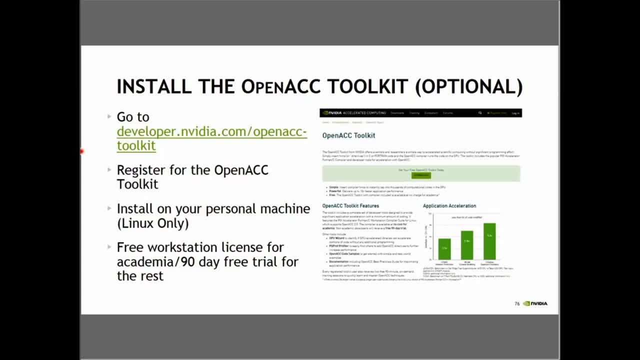 three months. if you're interested in teaching a similar course, please contact me or we'll help you out and give you more resources and materials to do so. okay, let me check if there are more questions. okay, uh, Jerry, there's one question about that again. could over MPI and GP direct, or you already answered. 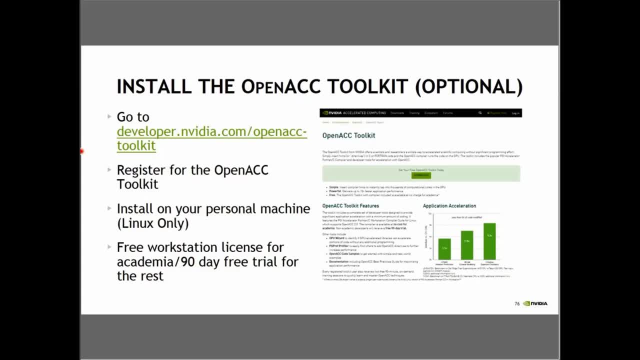 that's no right, never mind. okay, let's see if there are more questions in the last couple minutes and if not, I'm going to wrap it up. and another resource for you guys is exceed is actually in a partnership with Pittsburgh Super Computing Center. there are performing open ECC workshops and it happens three times a year and the next 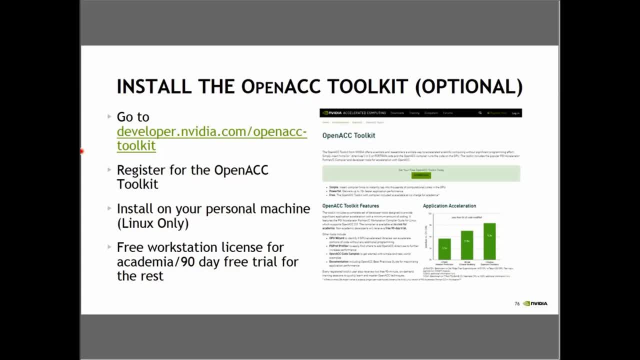 one will be mid-june and it will be open MP and open ECC combined. it's a three-day bootcamp. again, you're welcome to join. anyone is free to join. they don't have any limitations, I believe, and its workshop is designed to work on multiple sites, so they have about 12 or 13 different sites where people can. 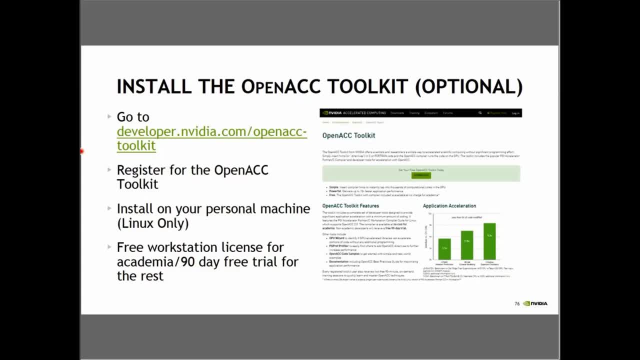 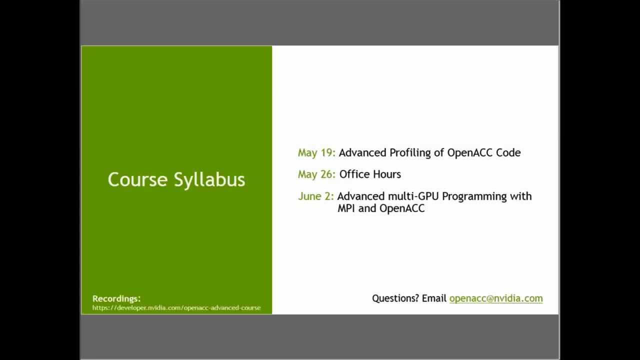 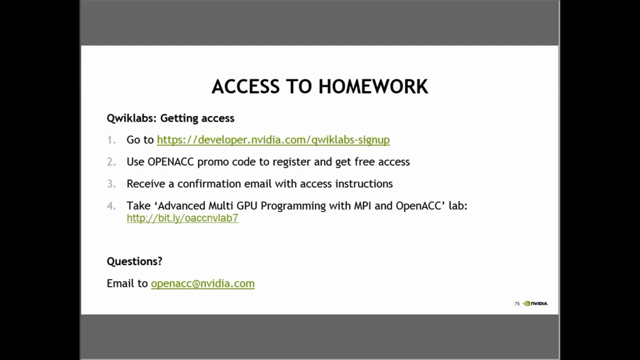 attend their workshop live okay. with that said, I believe we will wrap it up. thanks a lot for joining, really appreciate all your questions and attendance is really happy to see that this is something helpful that we're doing. and one more time, there are the link for their homework. and don't forget to register to get a 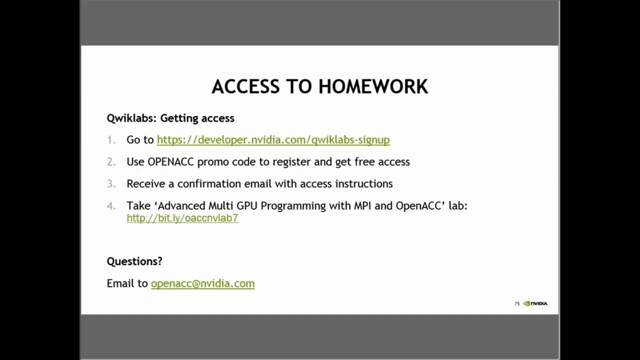 free credits to use their labs. if you don't have enough, please send out email. we will be happy to give you more credits to complete the homework. thanks all for joining. recording will be available later this week. thanks again and see you next time.